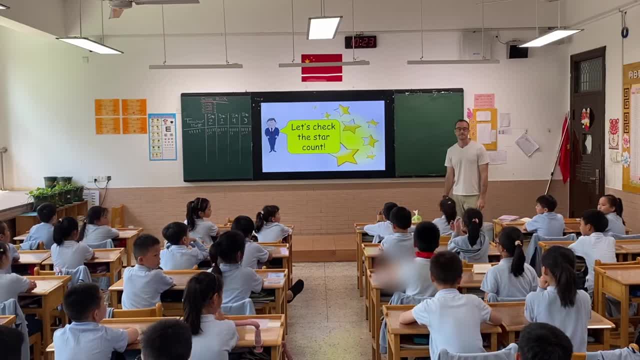 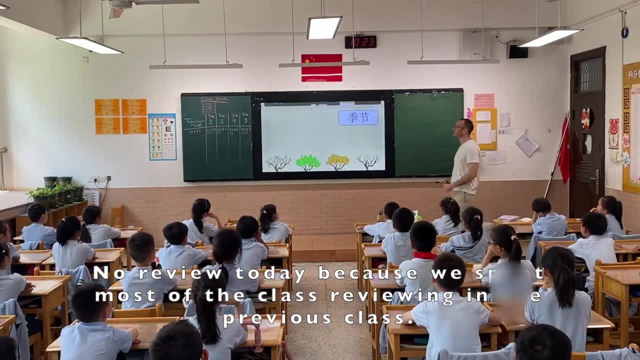 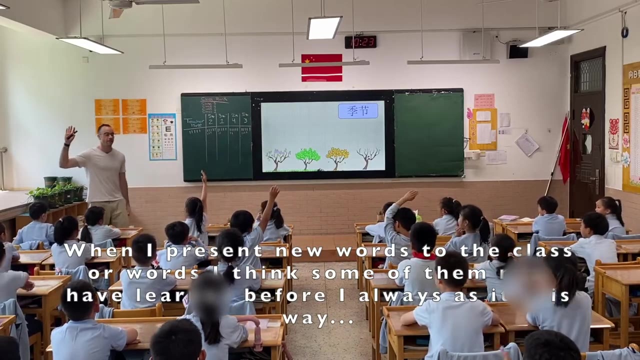 Team four: how many stars do you have? We have two stars. Good job, Alright, everyone. let's work, Let's work. Today, we're going to be learning about these. If you know how to say this in English, please raise your hand. 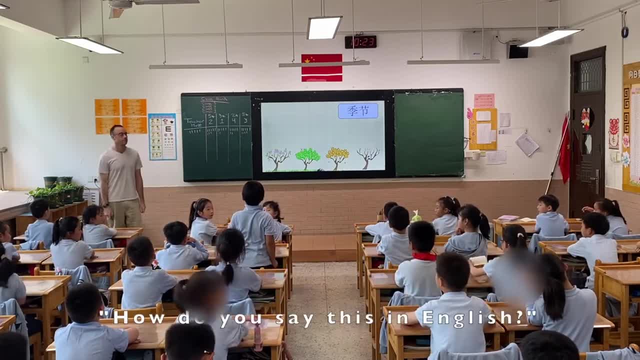 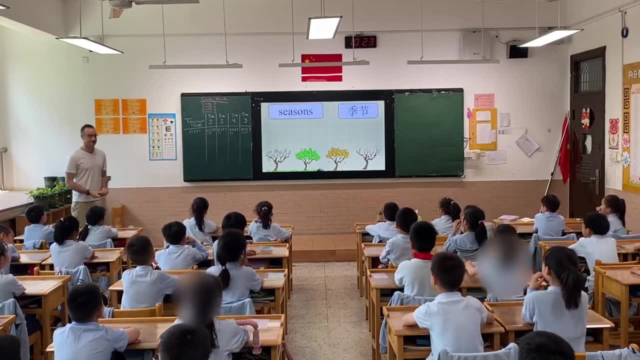 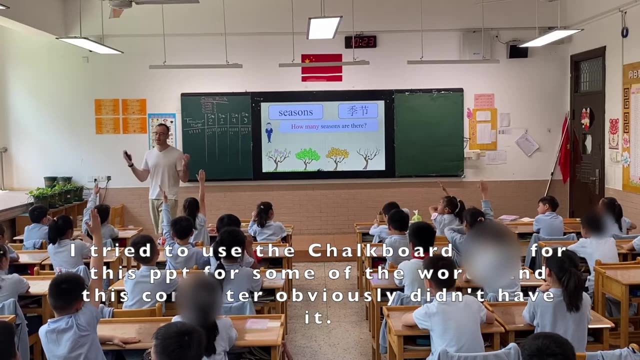 How do you say this in English? Weather, No, not weather. Good guess, though, not weather. Seasons, Good, everyone. seasons Seasons, Seasons, Seasons, Seasons, Seasons. How many seasons are there? How many seasons are there? 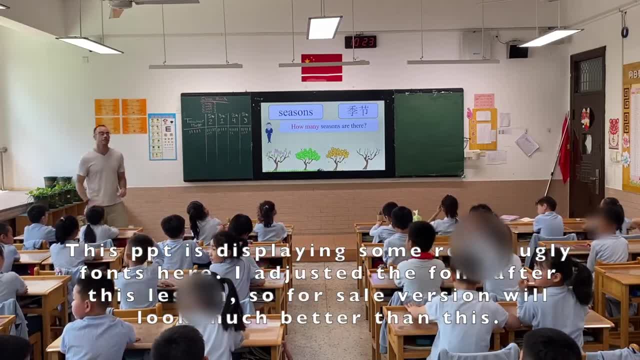 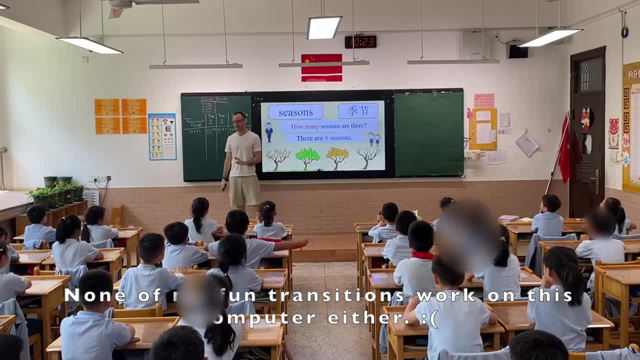 How many? Yes, how many. There are four seasons in one year. Good, Very good, Everyone together. There are four seasons. Good, There are four seasons. Okay, let's see How do you say this word: Breeze. 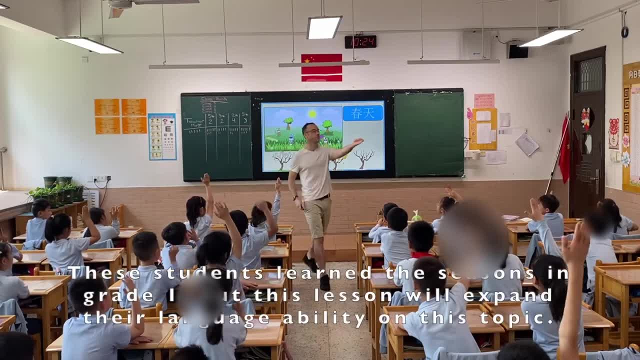 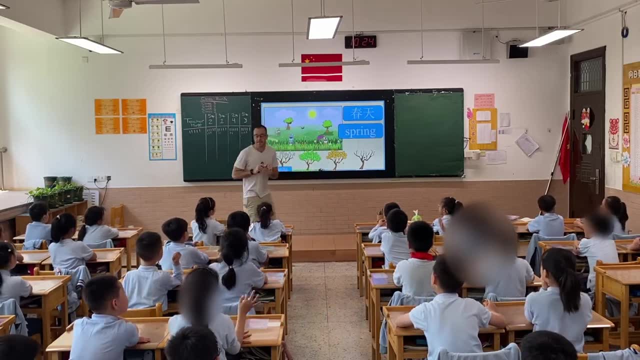 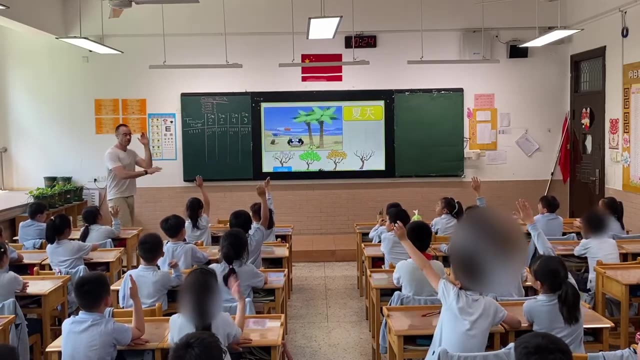 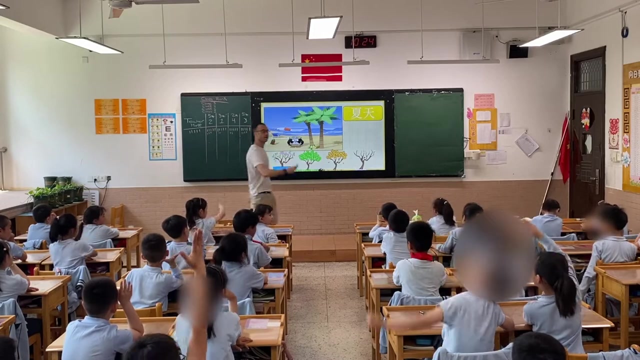 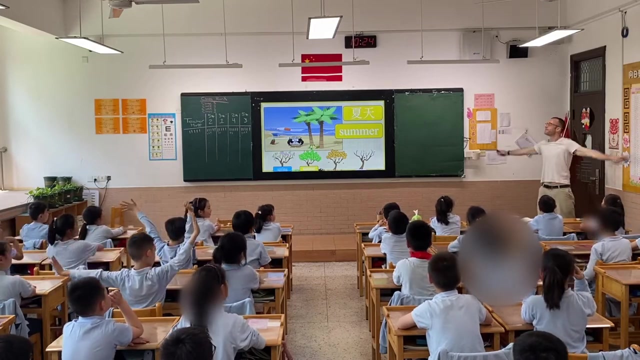 Breeze your hand. Breeze your hand, if you know. Breeze your hand. How do you say this in English? Breeze Go everyone. Spring Spring, Spring, Spring Spring, Very good, Very good. Next one, How do you say this in English? Raise your hand, if you know, In the front here, Not sunny Close. Yes, how do you say it? Go everyone, Summer, Summer, Summer, Summer, Summer. 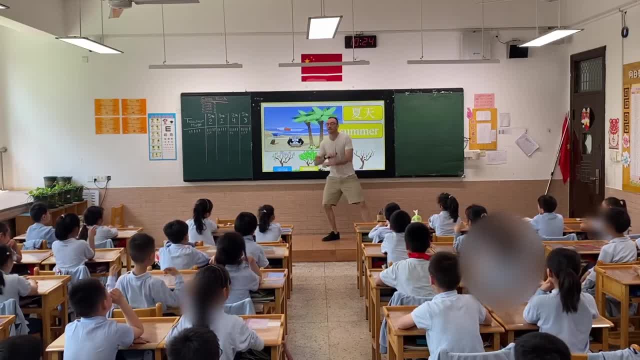 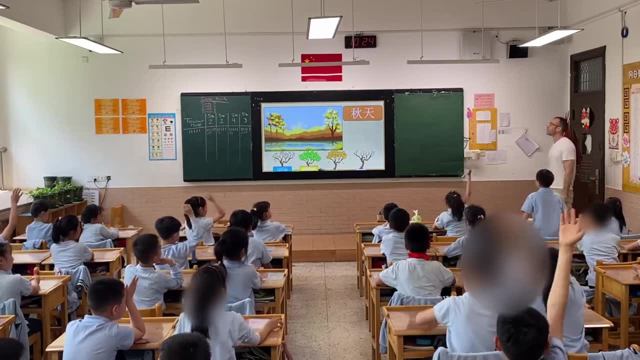 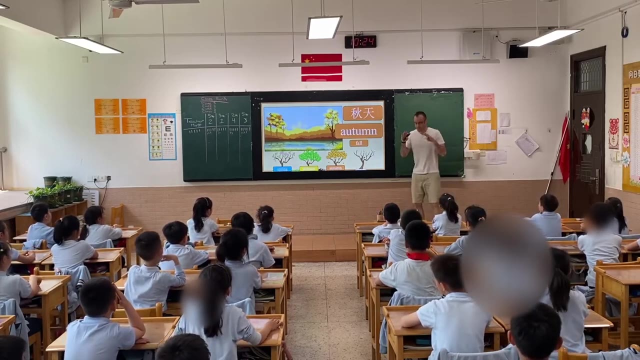 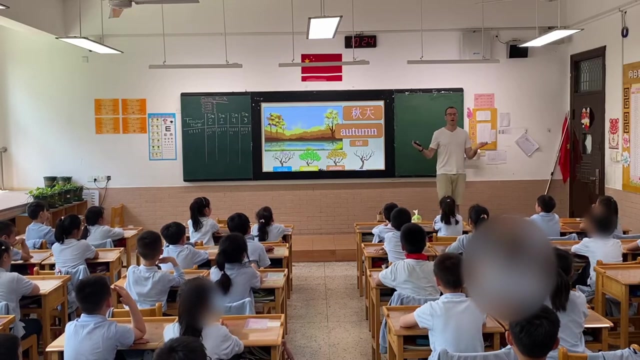 Very good. Spring, Summer, Summer, Summer, Good. How do you say the next one? Raise your hand if you know. Yes, Autumn, Good Everyone. Autumn, Autumn. There are two words. Fall. We can say autumn, Autumn, Fall, Fall, Autumn, Autumn, Fall, Fall. Why is it called fall? Why? Why do we call it fall? 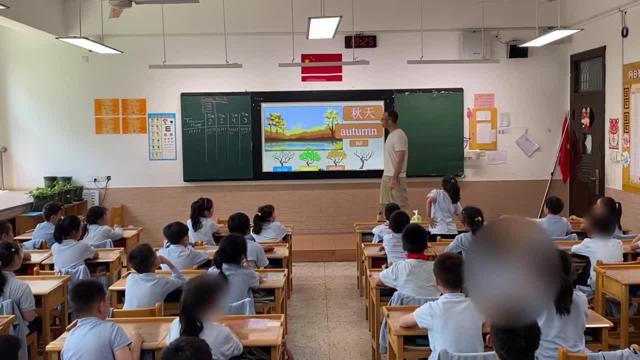 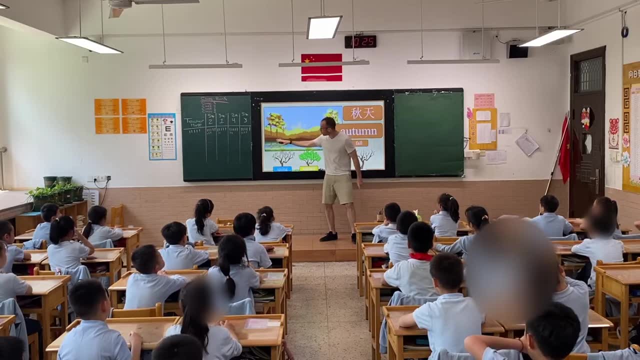 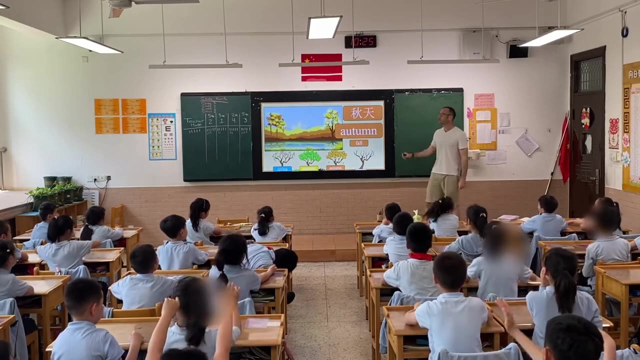 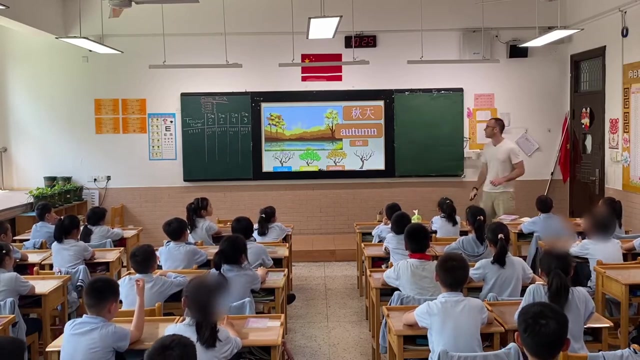 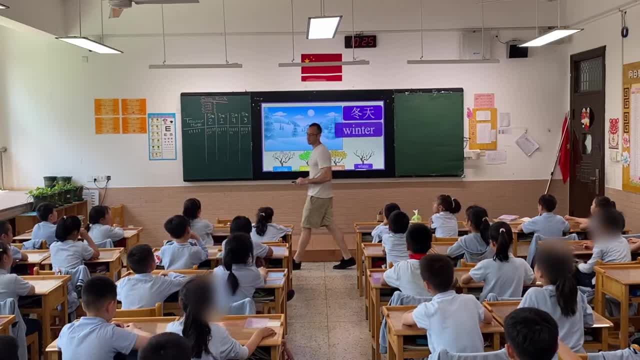 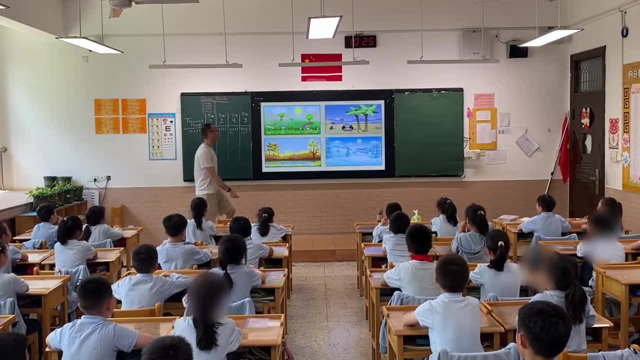 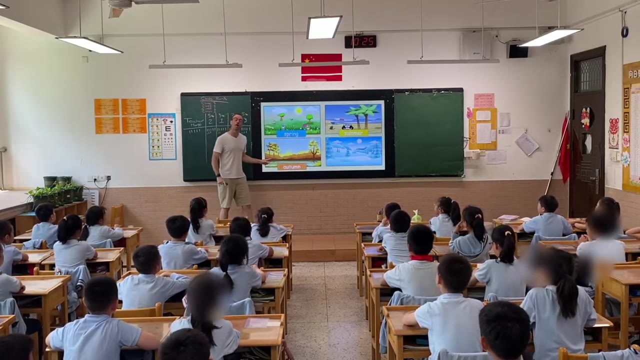 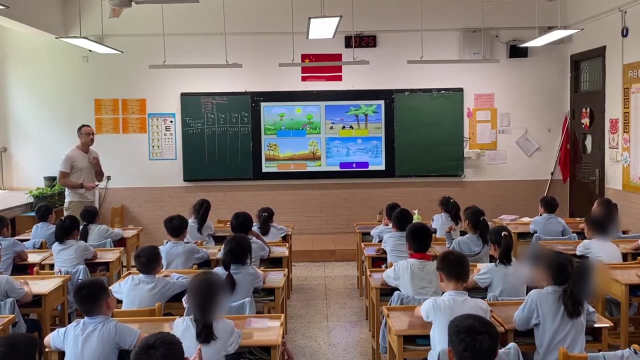 Yes, Winter, Good, Everyone. Winter, Winter, Winter, Winter, Winter, Winter. Let's say them all one more time again: Everyone together. How do you say it? Spring, Summer, Awesome Four. Fall And Winter- Excellent job. Now we're going to play the quick say game. Teacher Matt will say the season, You say the number. Okay, 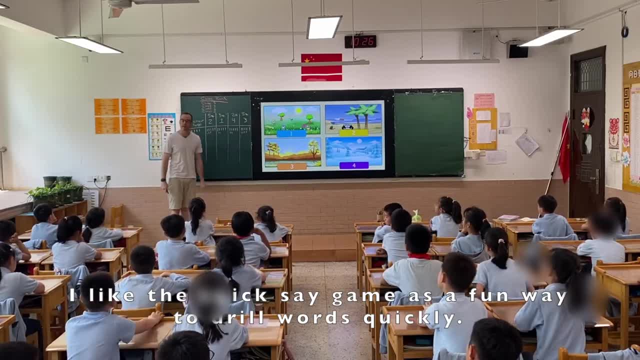 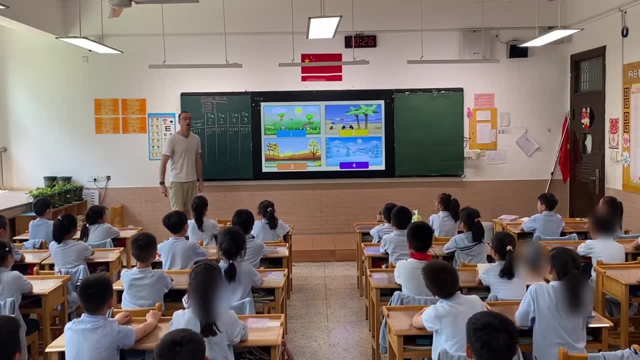 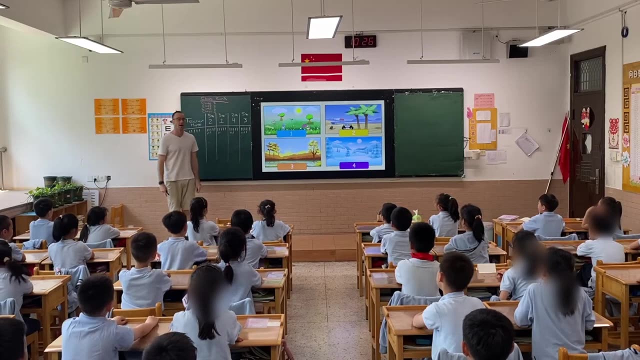 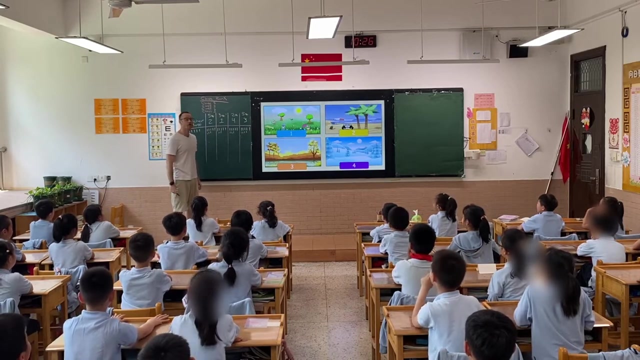 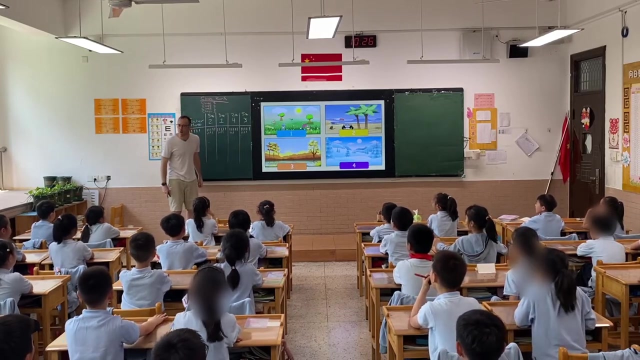 If you're very, very fast, I will give you 13 points. Are you ready? Yes, Summer, Very good job. Winter, Spring, Spring, Autumn, Autumn, Spring, Autumn, Spring, Fall, Fall, Fall, Fall. 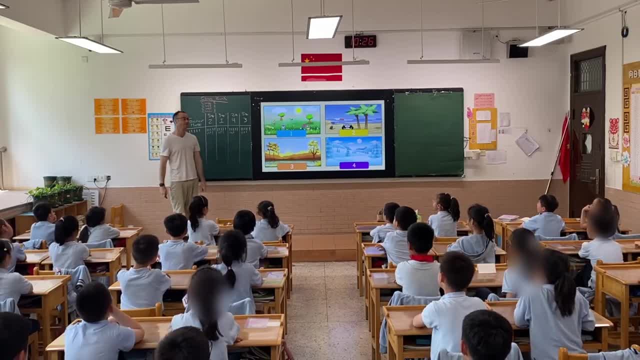 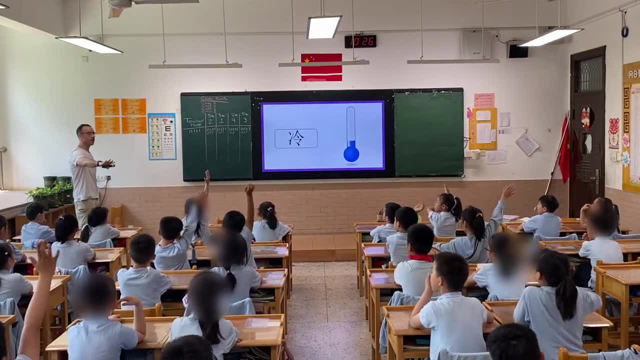 Good job, very, very, very good, good job. Teaching part two. teaching part two: Take it off, raise your hand, take it off, raise your hand, take it off, raise your hand. Okay, watch, How do you say it. 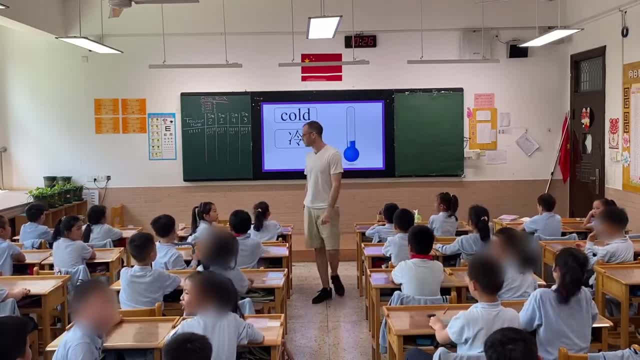 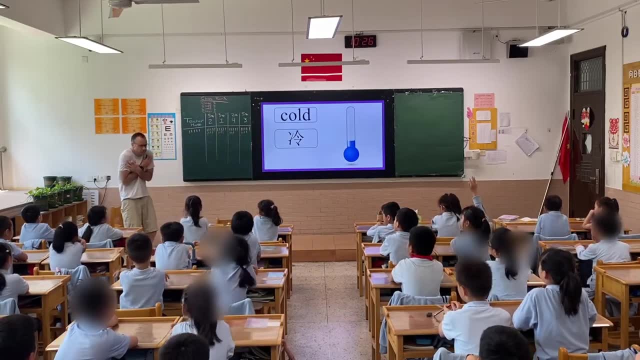 Yes, Very good. Everyone cold, Cold, Cold, Cold. What's the action for cold? What's the action? Go ahead, everyone, Cold, Cold. Everyone cold, Cold, Cold, Cold, Cold. Is it today cold? 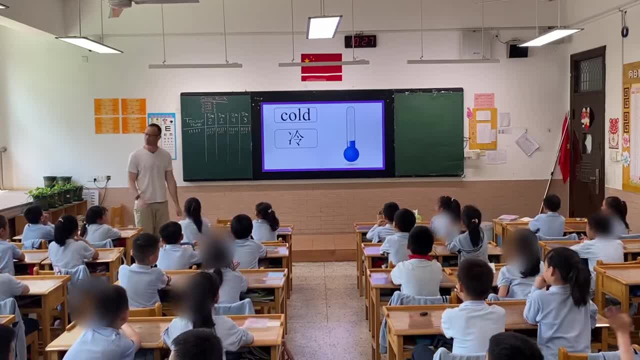 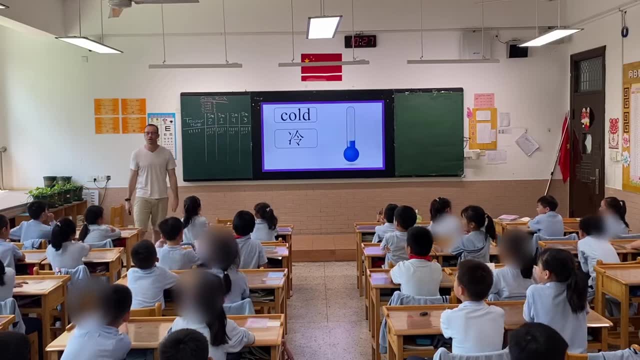 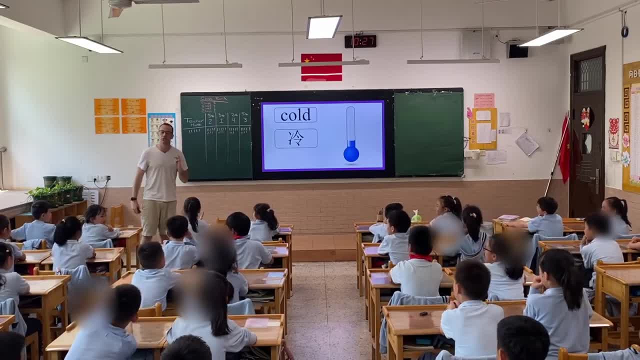 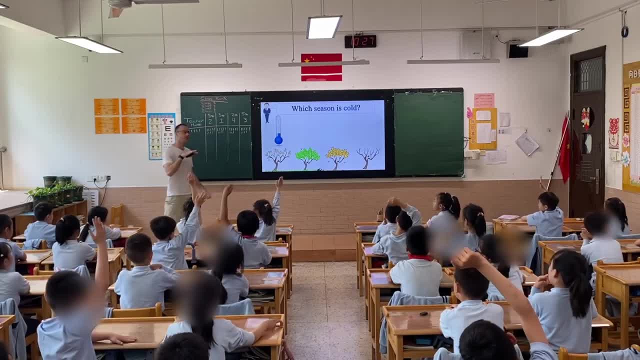 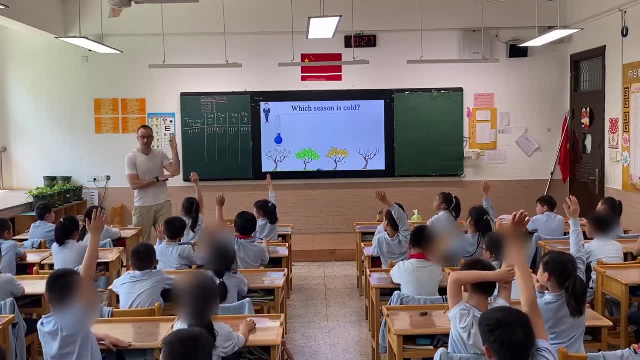 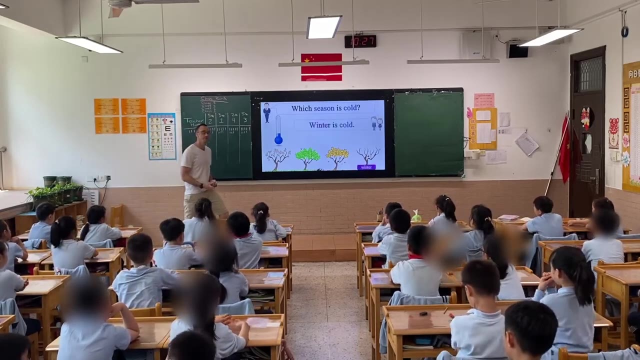 So which season is cold? Everyone together. Which season is cold? Which season is cold? Yes, which season is cold? Yes, Winter is cold. Perfect, everyone. Winter is cold. Winter is cold. Which color is this Winter? 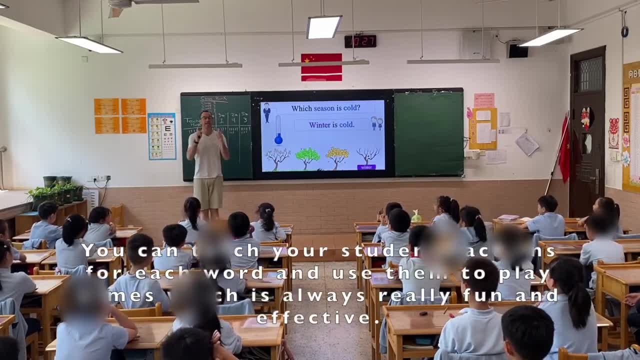 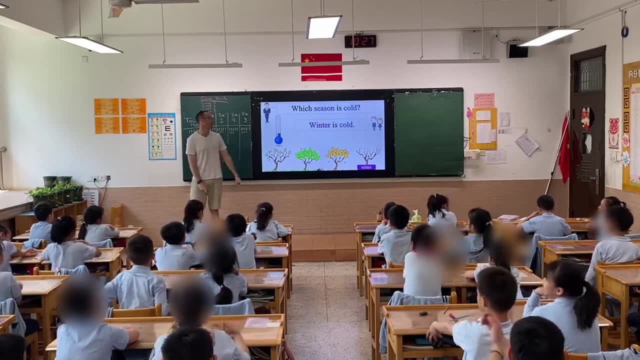 Winter It's, It's Cold, Cold Winter. Winter It's It's Cold, Cold. Very good, Excellent. How do you say this in English? Raise your hand, if you know. Raise your hand. Raise your hand, if you know. 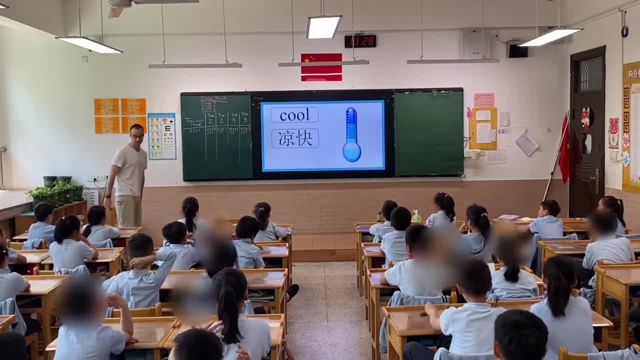 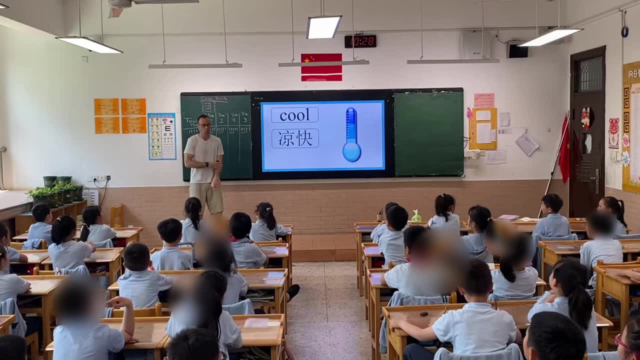 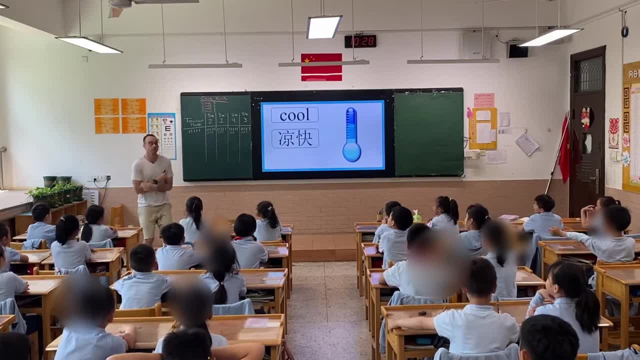 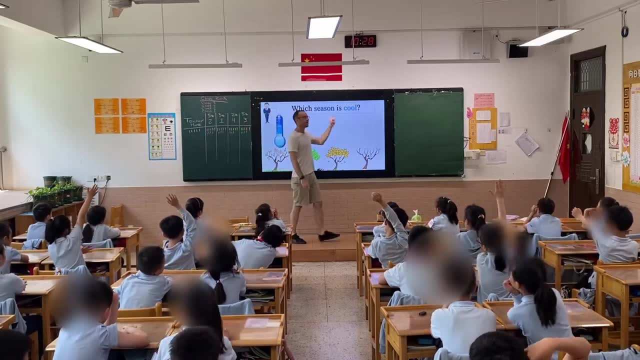 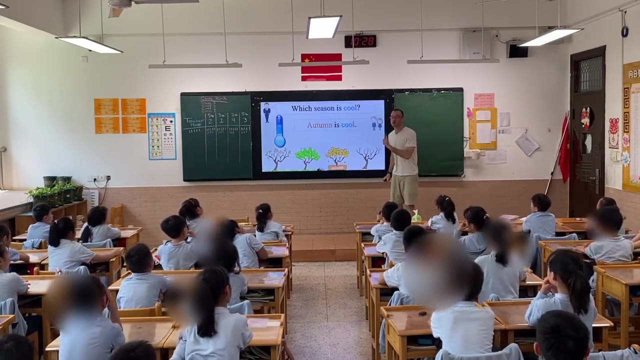 Cool, Good job. Pool, Pool, Pool, Pool, Pool, Pool, Pool, Cool job Everyone together. Which season is cool? Yes, Cool, Cool, Cool, Good job Everyone. you can say: Fall is cool, or? 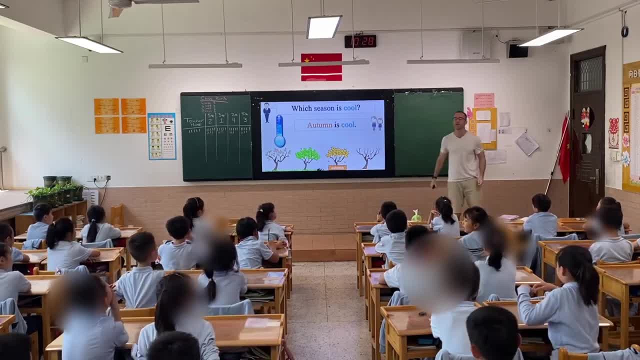 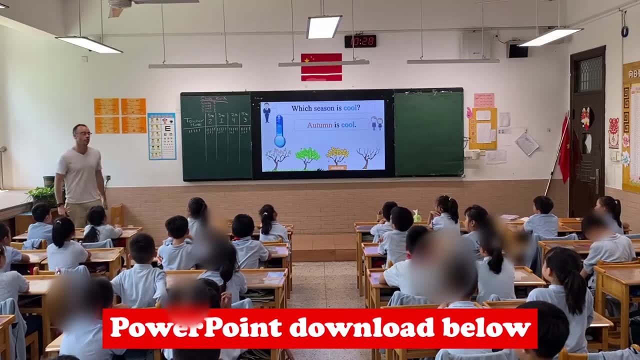 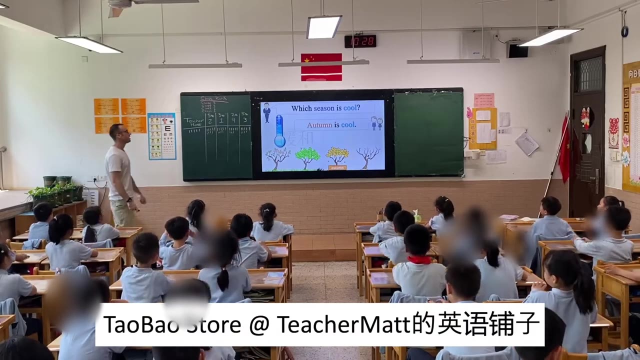 Autumn is cool. All are correct, Everyone. Autumn, Autumn is Is Cool, Cool, Very, very, very, very good. Also, the action is this Autumn, Autumn is Is Cool, Cool, That's right. 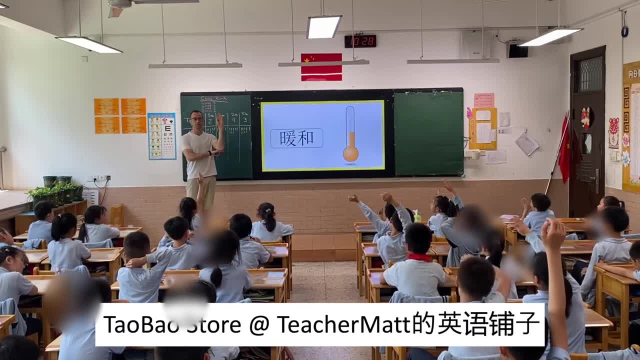 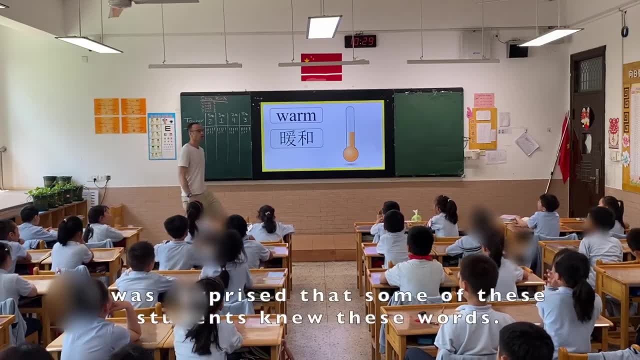 Next one. How do you say it in English? Did you know the script? Did you know the script? Yes, Warm, Great, Good job Everyone. Warm, Warm, Warm, Warm, Warm, Warm Warm. We use one hand like this: 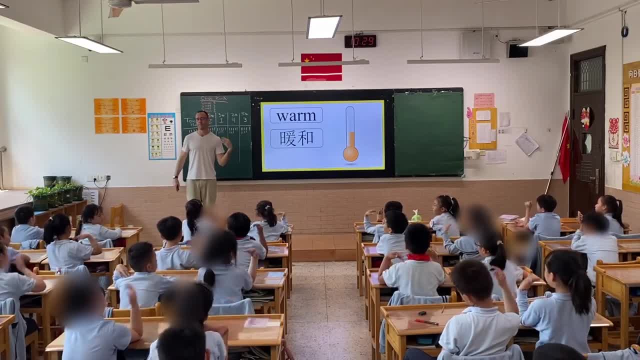 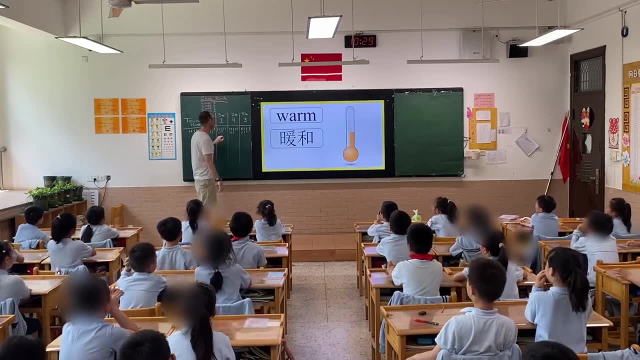 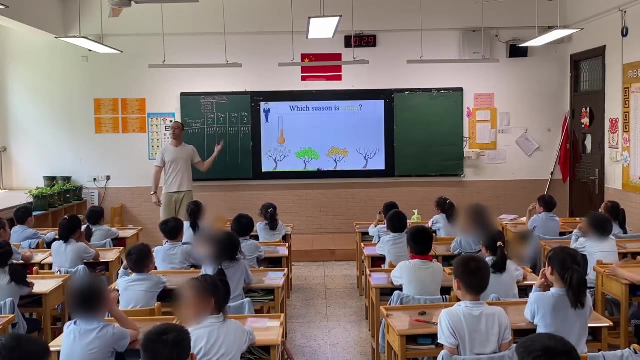 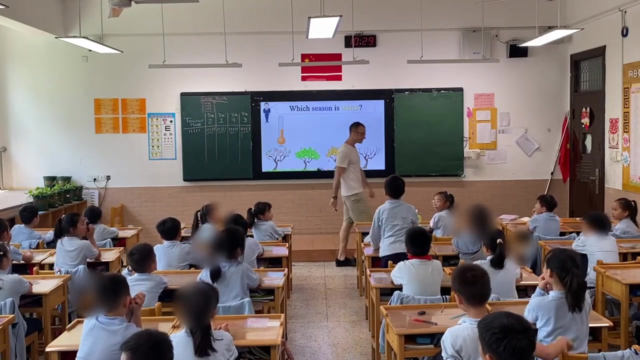 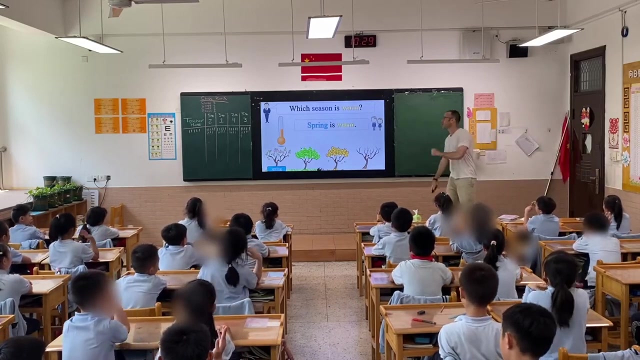 Warm, Warm, Warm, Warm, Warm, Warm, Cool, Cool, Warm. Everyone together хочу is warm. Yes, Very good job. Everyone scream Praise: is war Good? Last one, Raise your hand if you don't. 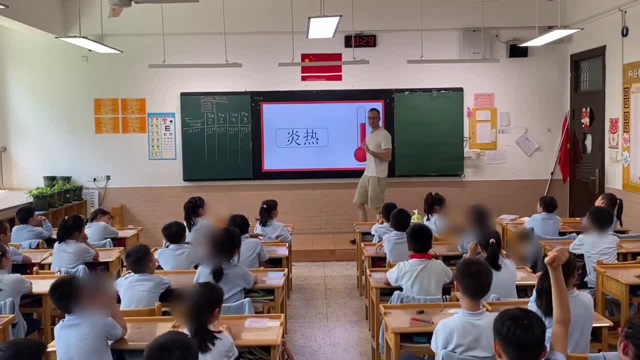 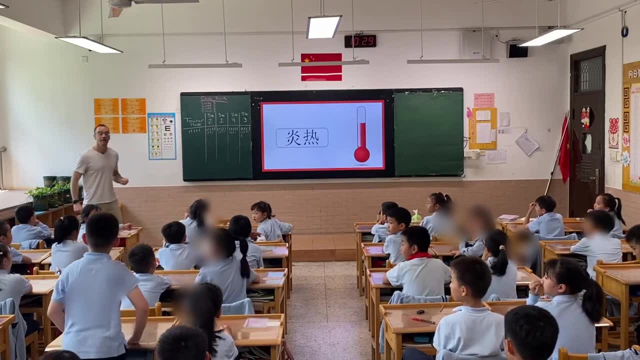 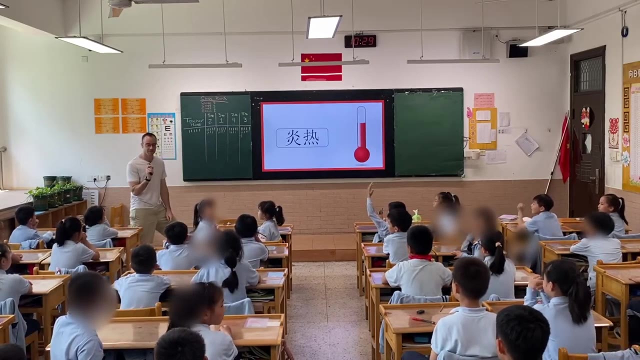 Raise your hand. if you don't, Hot, Hot, Let's make it even. How do you say Hot? Do you know Hot is okay. There's another word we say together. Do you know? Hotest, Not hottest, Hot, Hotest. 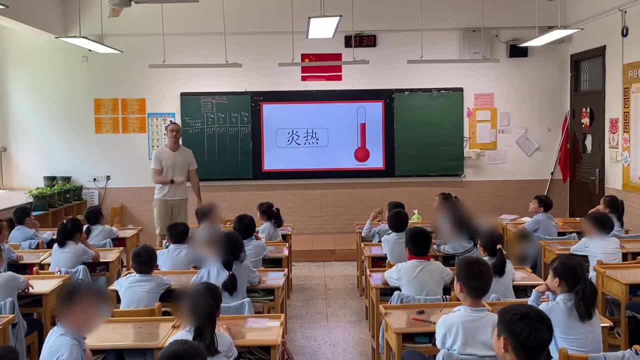 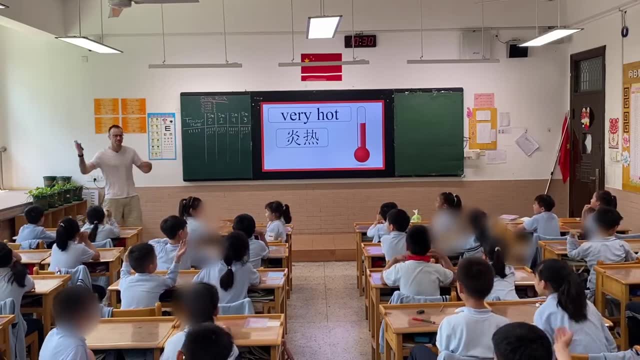 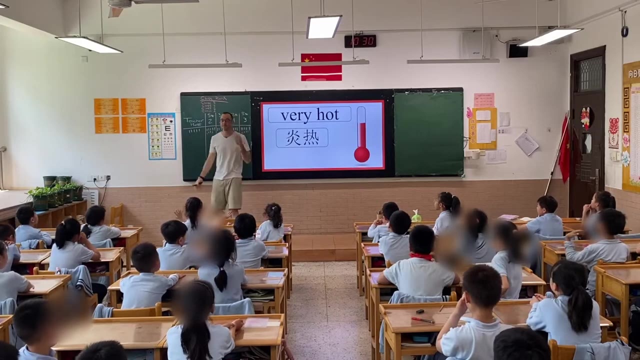 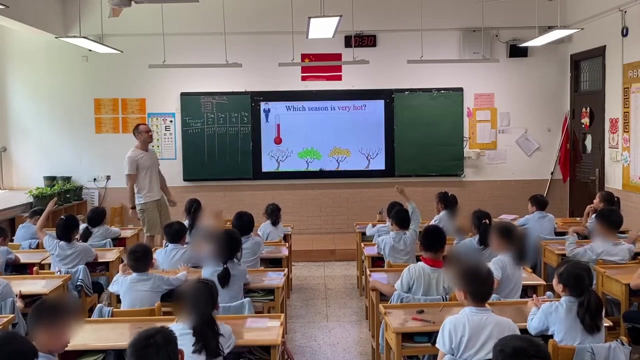 Look at my mouth: Hotty, Good job Everyone. Very hot, Very hot, Very hot. Hot is okay too. You can say hot, But today we're saying very hot, Very hot, Very hot. Everyone. This season is very hot. 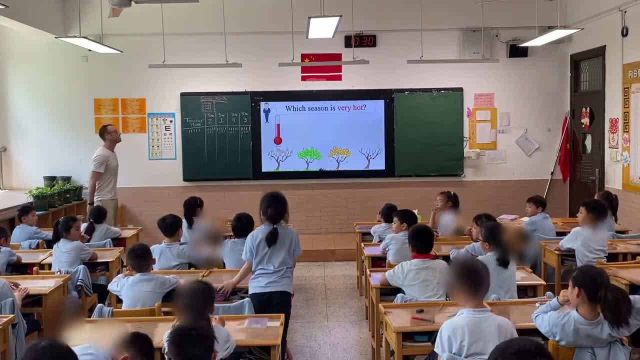 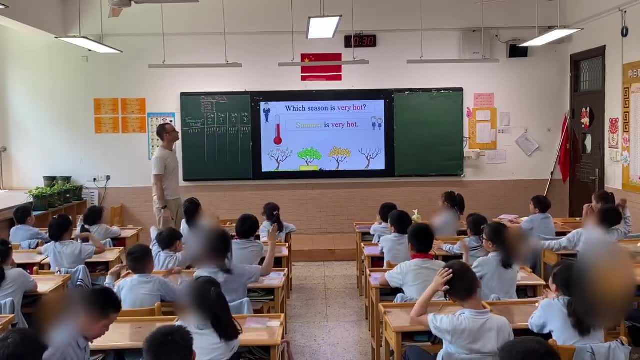 There's only one season left. Yes, Summer is very hot. Good, Everyone, Summer, Summer is hot, It's hot, It's hot, Very hot, Very hot. Good, Let's say them all again. Let's say them all again: Everyone Together. 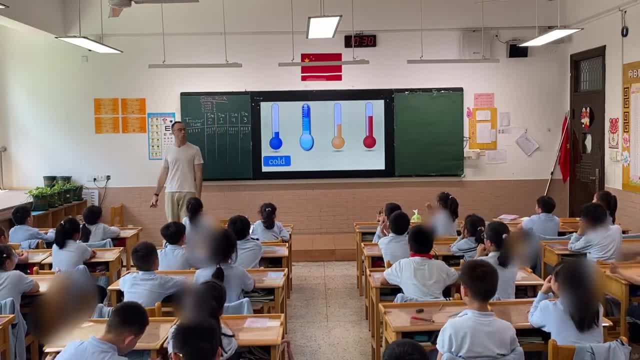 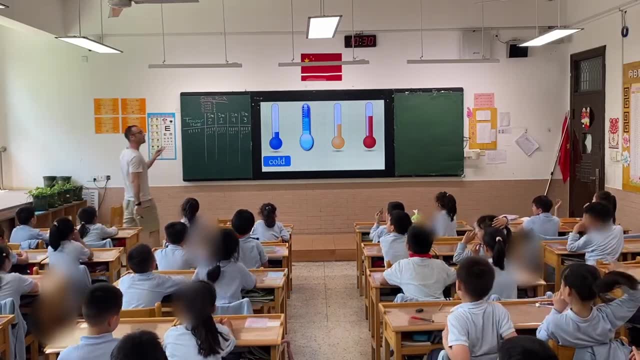 Cold, Cold, Cold, Cold. This season is cold. Who can tell me in a sentence which season is cold? Yes, The winter is cold. Good Everyone. Winter is cold. Winter is cold. Next one: Cold, Cold, Good Everyone. 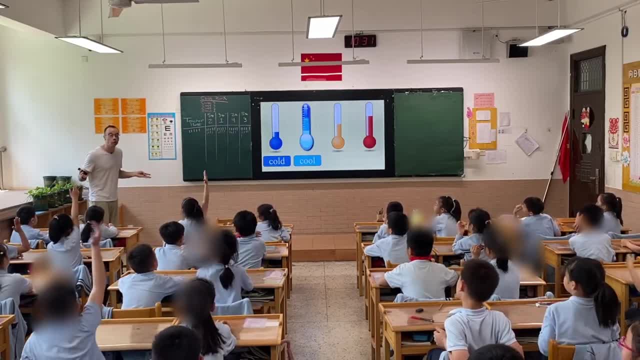 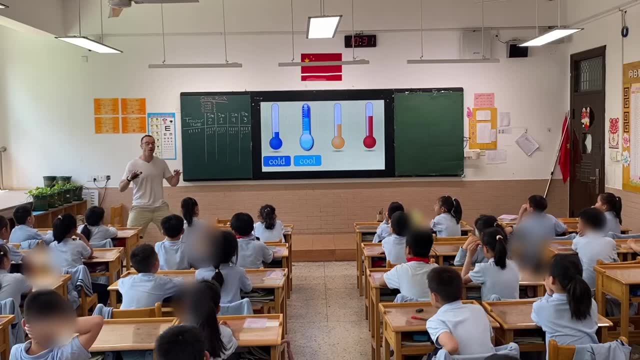 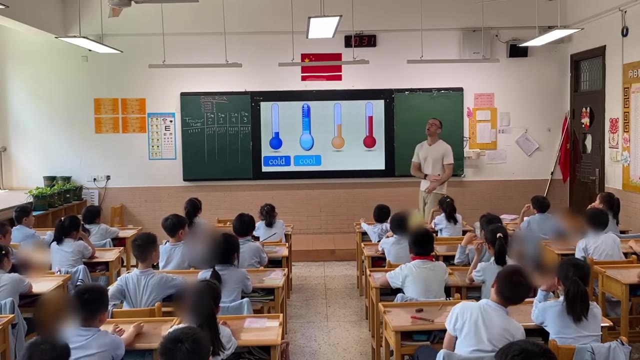 Next one: Cold, Cold, Cold. Next one: Cold, Cold. Who can tell me in a sentence which season is cold? Yes, The spring, The spring. The spring is cold, Very good. You can say the fall, Or The autumn, The autumn. Next one: Awesome, Awesome, Is Is Cold, Cold. Good job. Next one. 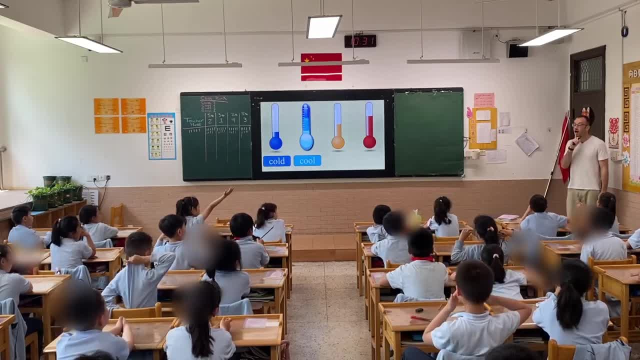 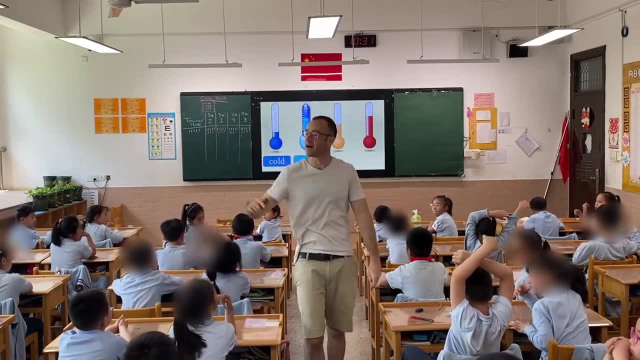 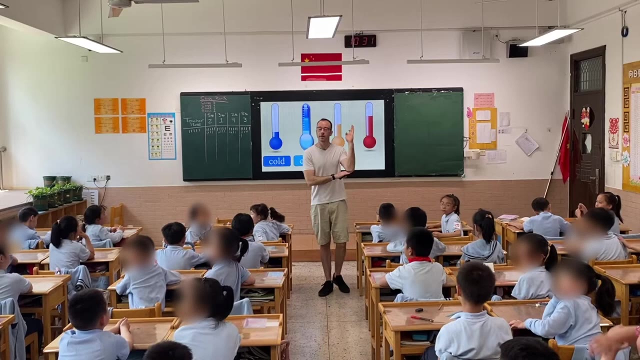 Oh, The next one: Hot, Hot, Hot, Our hot, Your time, Your time, All right In the back There. This point, Yes, Yes, How do you say Who can help him? Who can help him? 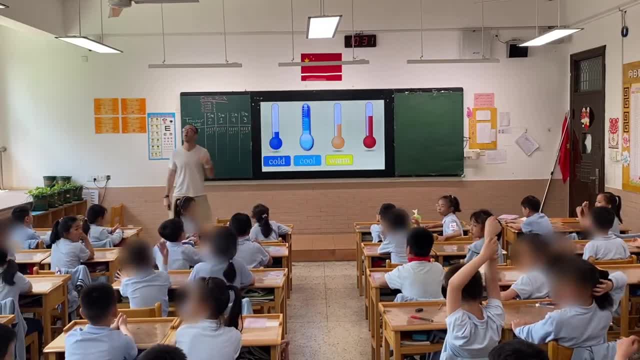 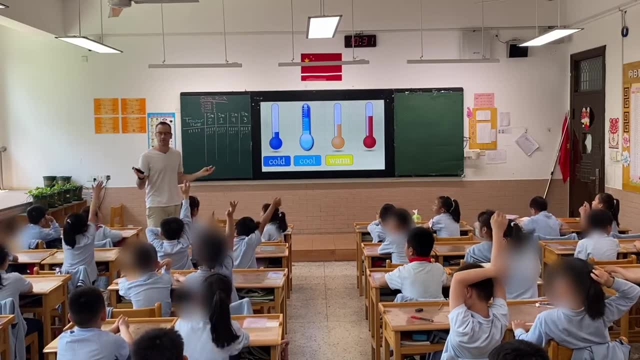 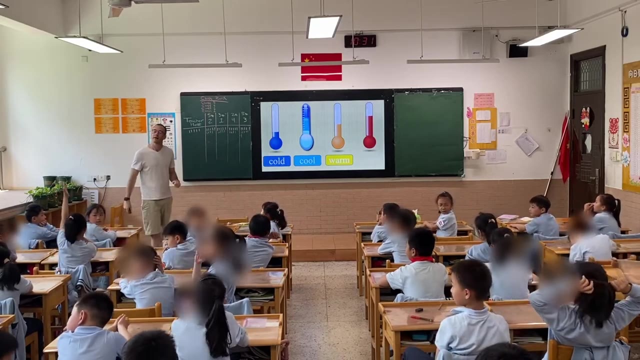 Yeah, Warm, Good, Warm, Warm, Warm, Warm, Warm, Warm. Which season is warm? Which season is warm? Yes, which season is warm? Spring, Good, everyone together, Spring, Spring, Spring Is warm. 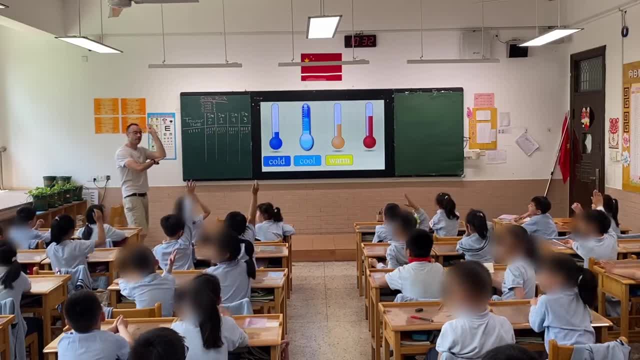 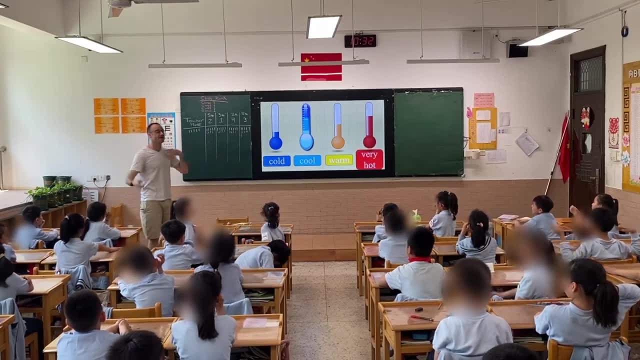 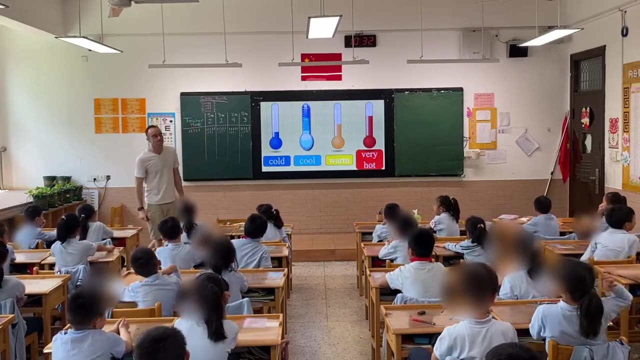 And the last one. That's the last one. Last one, Last one, All right, yes, Next one is very hot. Go everyone. very hot, Very hot. Look at my mouth, very, Very, Very Very. 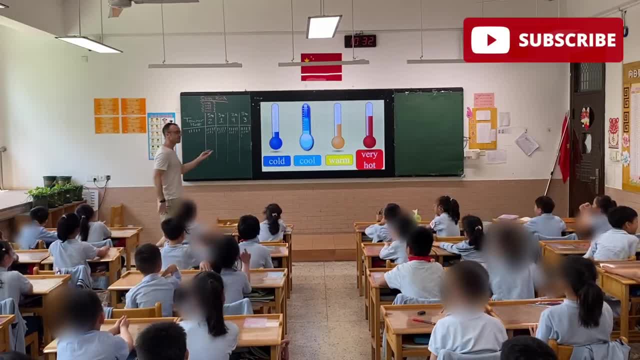 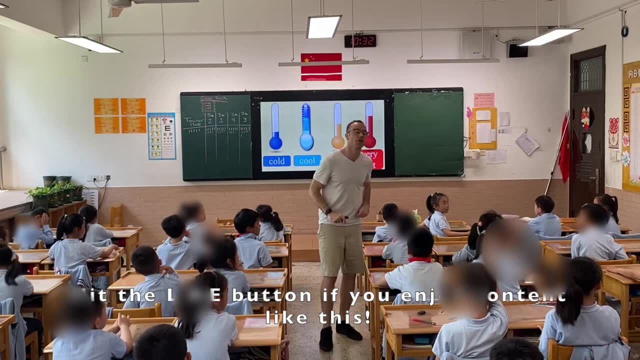 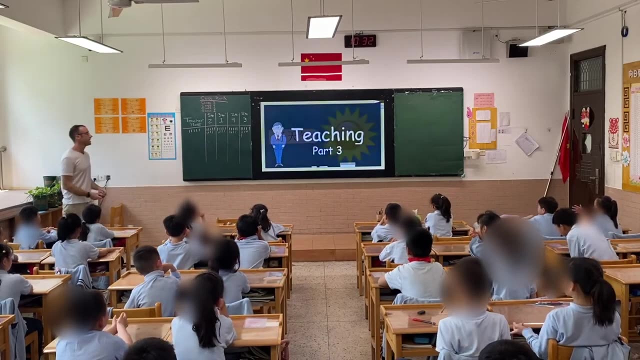 Very hot, Very hot. Which season is very hot? Which season is very, very, very hot? Yes, Very, Very Good. summer is very hot, Very hot. Good job, Let's go to the next part. Next part: how do you say this in English? 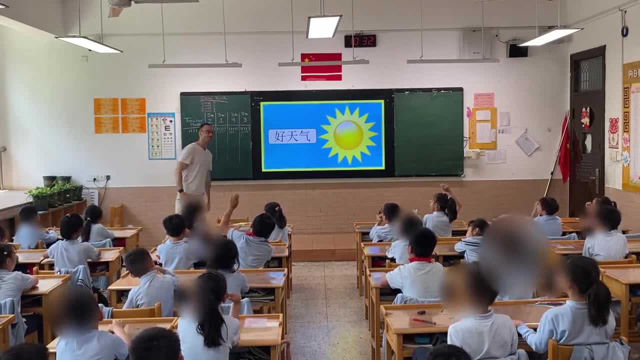 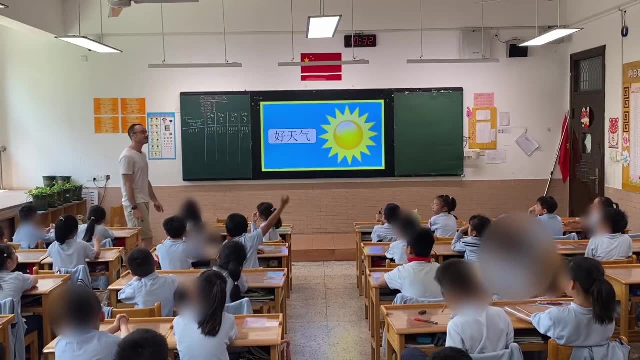 How do you say this in English? Very? How do you say this in English? Good, Okay, you can say good weather, You can say good weather. or we can say this word: nice, Nice, Nice, Nice, Nice When we talk about the weather. 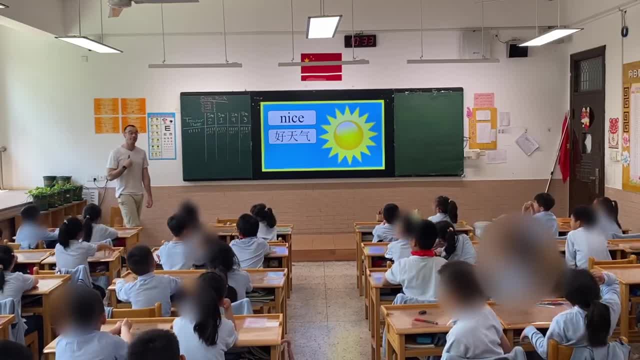 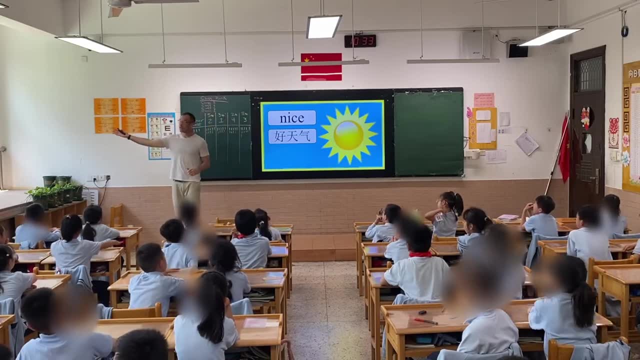 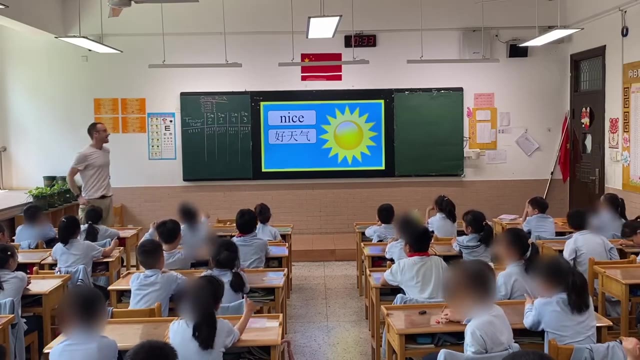 if I say, oh, it's nice outside, I mean it's nice weather outside. okay, Today is nice. look, is it nice? Yes, it's very, very nice. Everyone say nice, Nice, Nice, Nice. 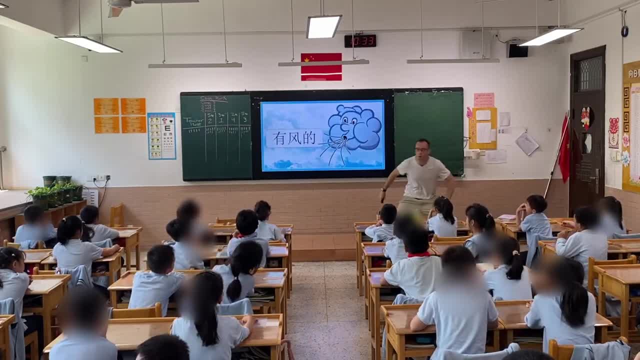 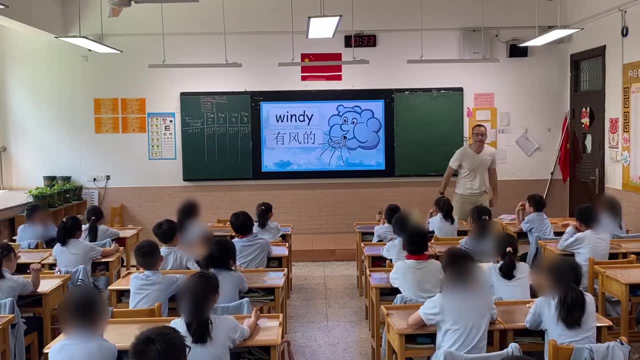 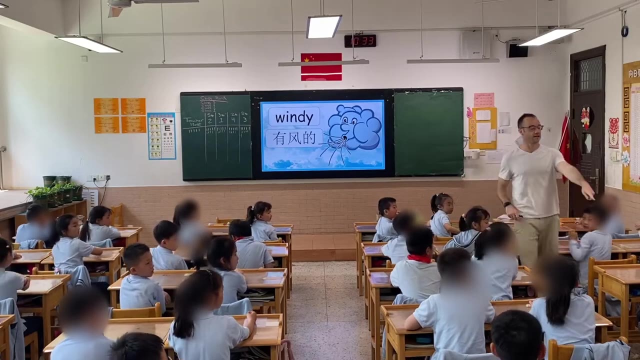 Nice, Nice. Next one: Windy, Oh, I hear it already. how do we say it? Windy, Oh, that's right. windy, Windy, Windy, Windy. Yes, Put your desk, please put your desk, put your desk. 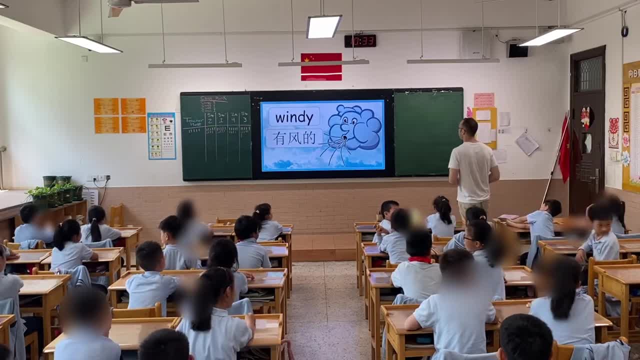 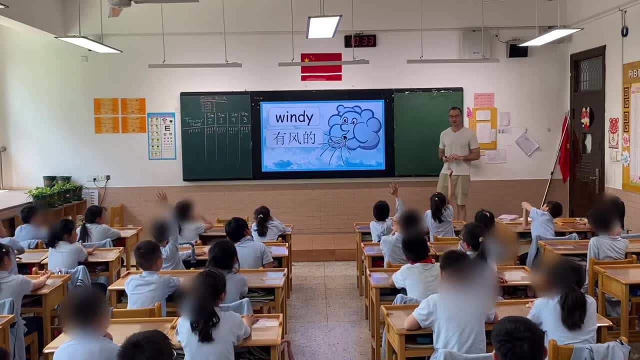 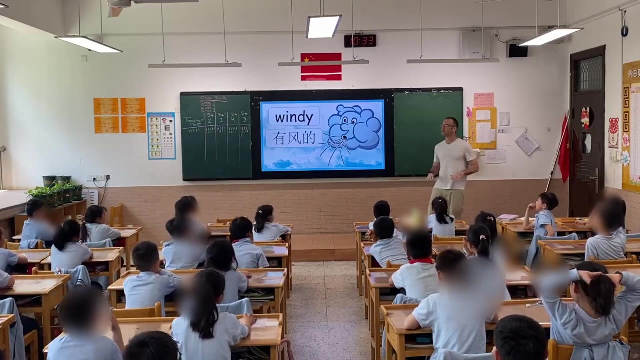 thank you good everyone. windy, Windy, Windy, Windy, Windy, Windy. Which season is windy, Which season is very, very windy? Yes, Good autumn, everyone. autumn, Autumn, It is very, very. 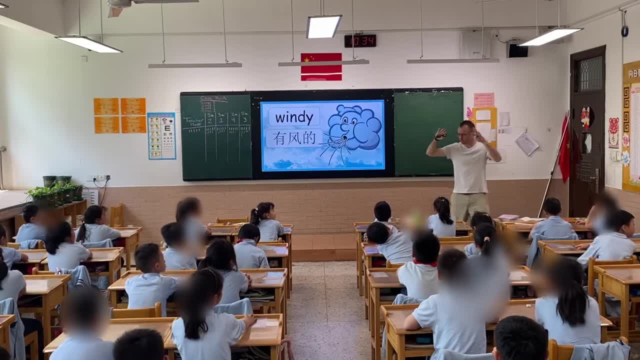 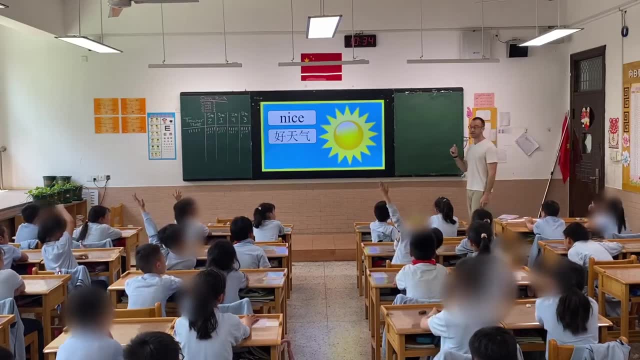 Windy, Windy, Windy. Good, so the leaves will fall down, that's right. Which season is very, very nice? Which season is very, very nice? Is the summer very nice? Yes, Oh, which season is very nice? 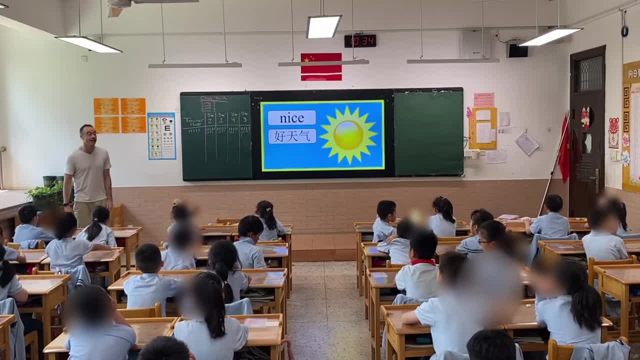 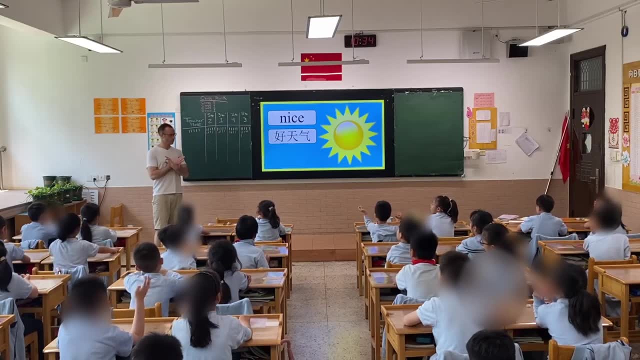 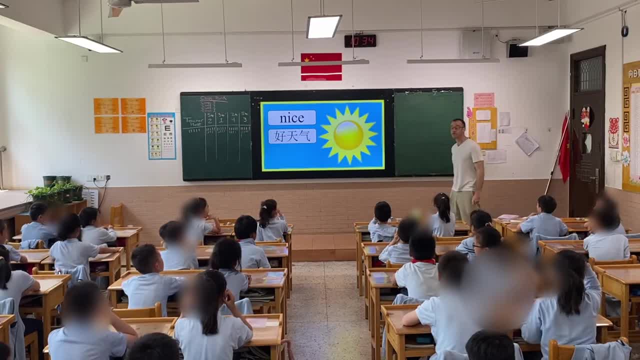 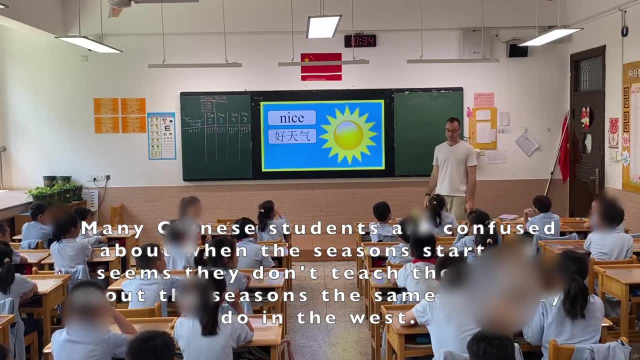 It starts in June. Summer starts in June. Summer starts in June. Right now it's May. It's May, It's still the Spring, Spring. Oh, In June, In June, Leave it. Summer begins Not yet. 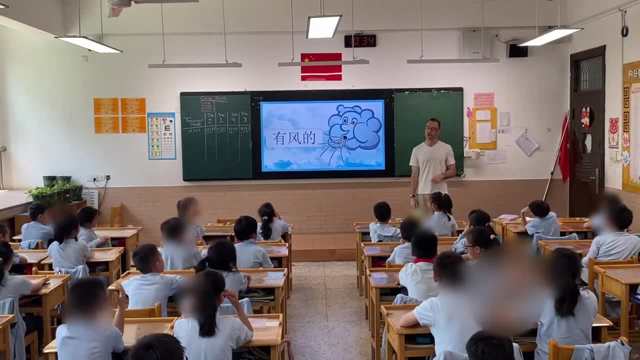 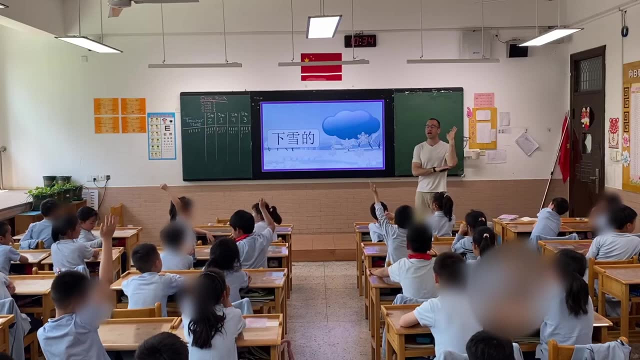 Not yet, Not yet Next one, Next one, Next one: Ready, Let's go Out. you say, yes, Go, go, Go go. Yes, very good, great, That's right. Such a really good thing to do this summer. 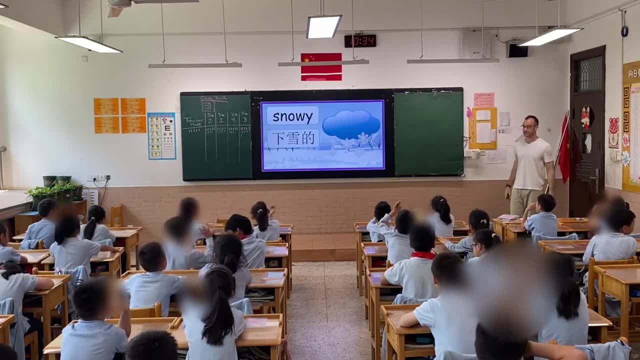 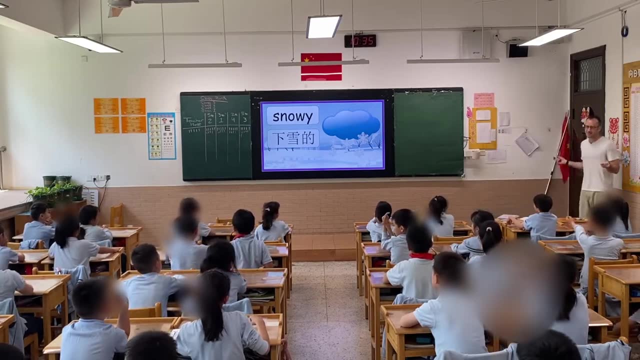 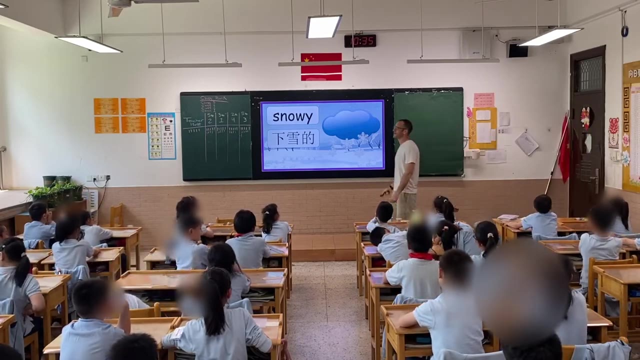 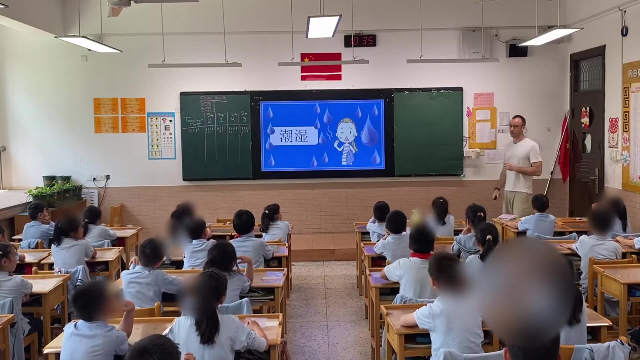 Good, Everyone. snowy, Snowy, Snowy, Snowy, Snowy, Snowy, Good job. Which season is very snowy? Which season? So we can see everyone together. Winter is snowy, Good job. And last one, Wet. Okay, We learned the word wet before. There's a better word to talk about the weather when it's like this. Do you know it? 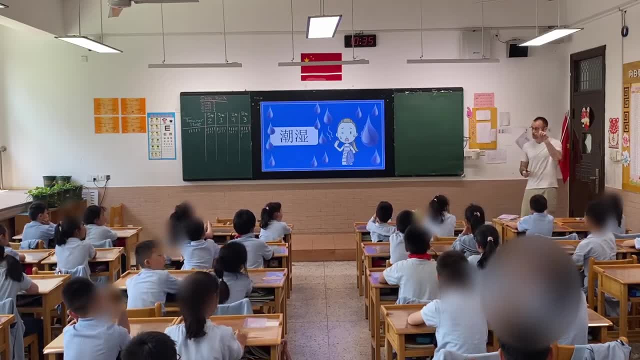 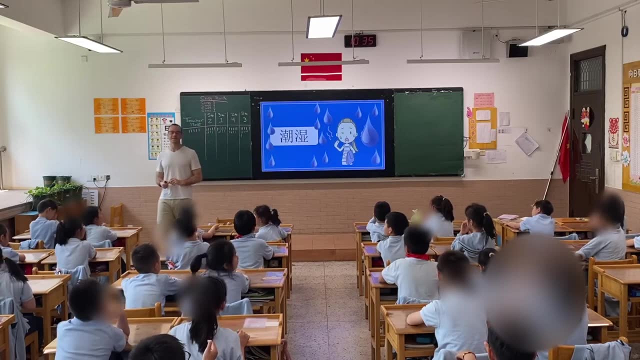 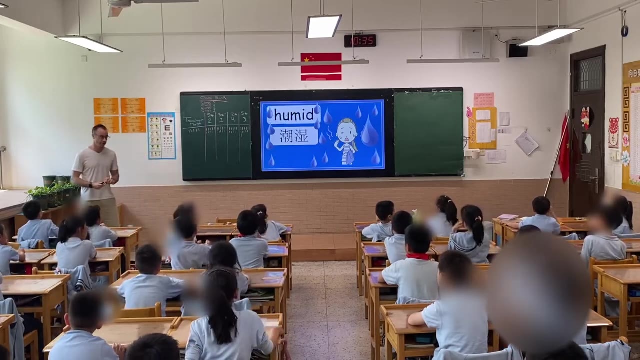 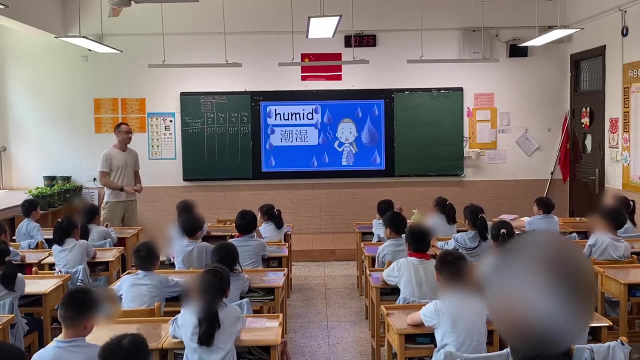 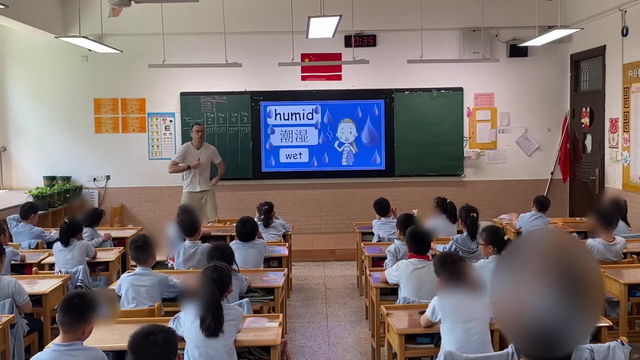 It starts with an H, What It starts with an H, H kind of word. You can say wet, but there's a better word than wet. We say it like this: Humid, Humid, Humid. Everyone humid, Humid. You can also say wet, Humid is a better word for this. Okay, Everyone humid, Humid, Humid. 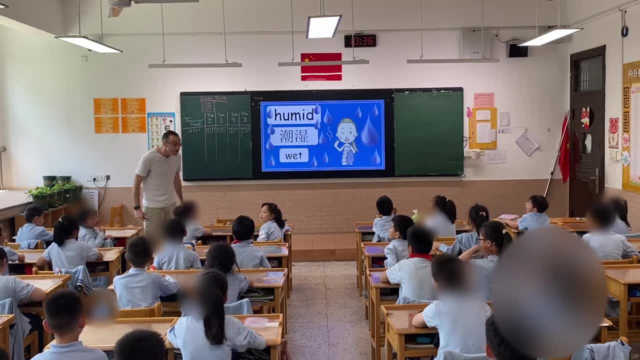 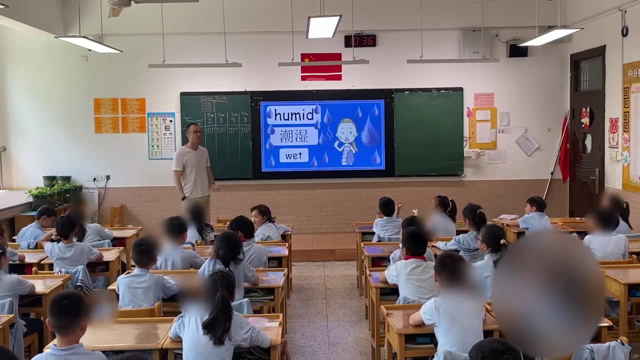 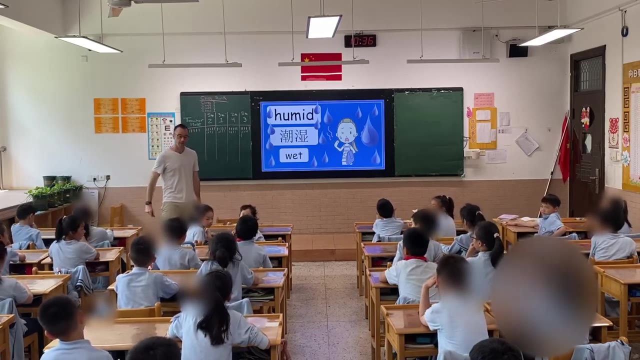 Do you like humid brother? Yes, Teacher Matt doesn't like humid brother, Because I'm very, very sweaty, Very, very sweaty, Very comfortable, Very sweat. Yes, I'm a little bit wet. A little bit is okay, A little bit is okay. 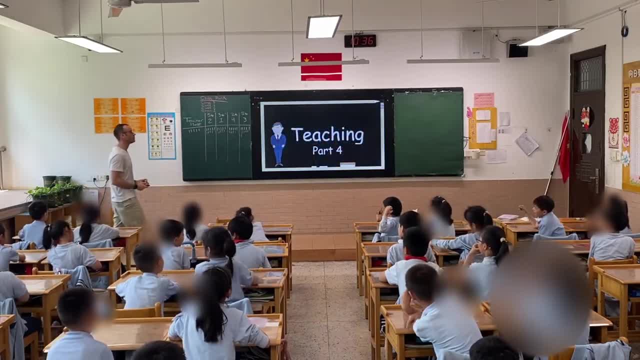 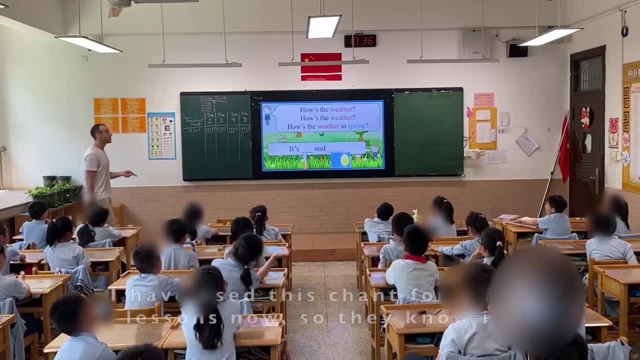 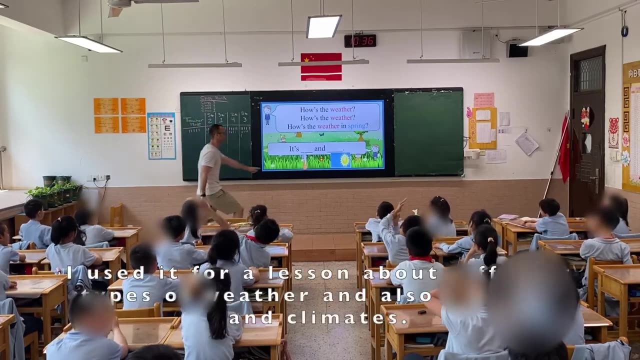 Let's move on. teach you part 4.. Everyone together: How's the weather? How's the weather? How's the weather in spring? Hmm, How's the weather in spring? There's two of them. You can say two blues here. 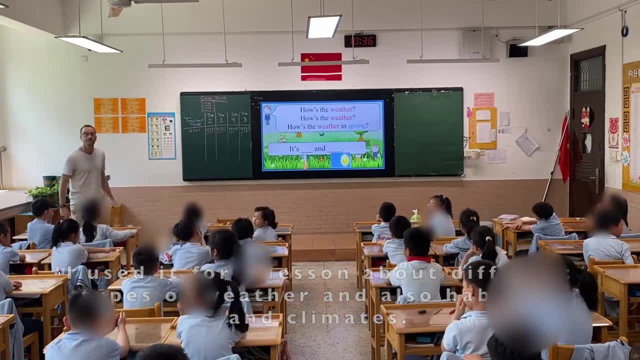 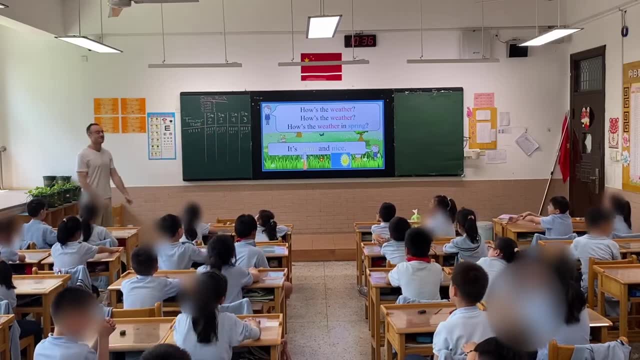 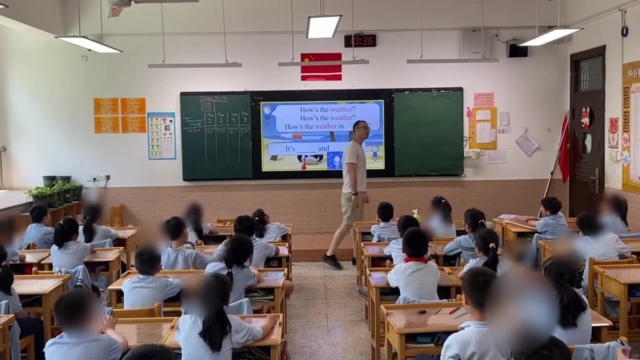 How's the weather in Spring? Yes, It's warm and nice. Good job Everyone. It's warm and nice, Good job, Very good, Very good, Everyone together. How's the weather? How's the weather? How's the weather in summer? 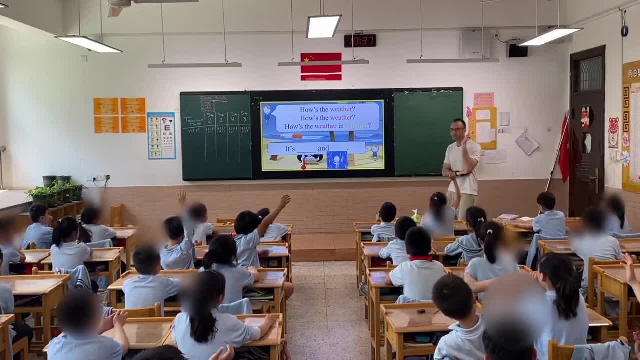 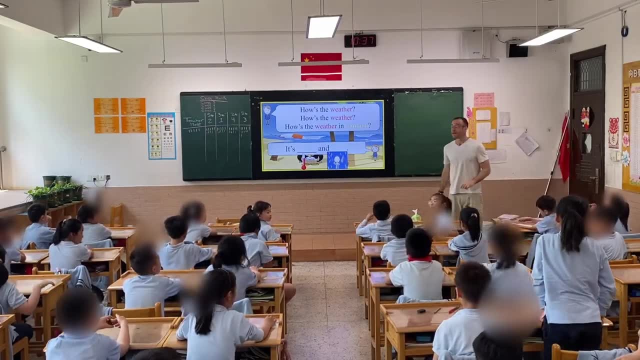 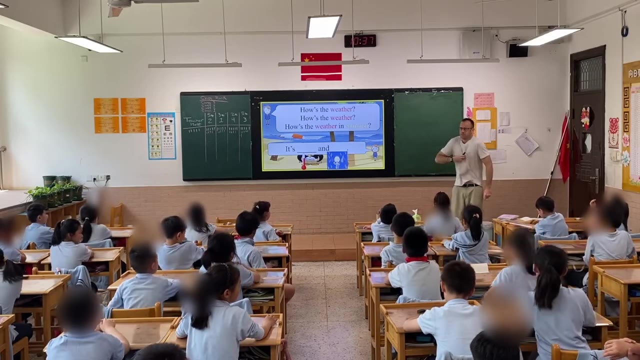 How's the weather in summer? How's the weather in summer, Anyone different? How's the weather in summer? Alright, yes, How's the weather in summer? Okay, Wet or Humid, Everyone humid, Humid, Humid. 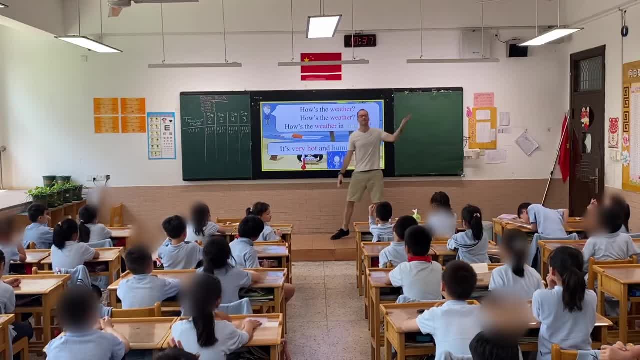 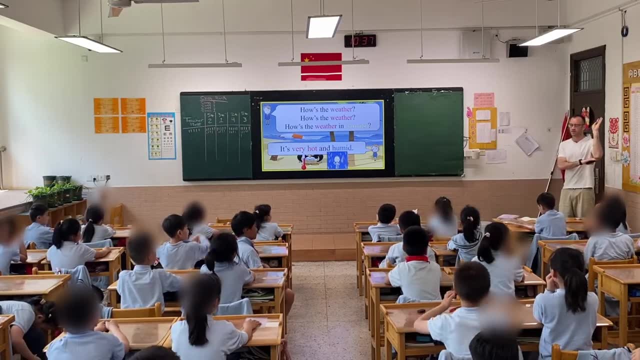 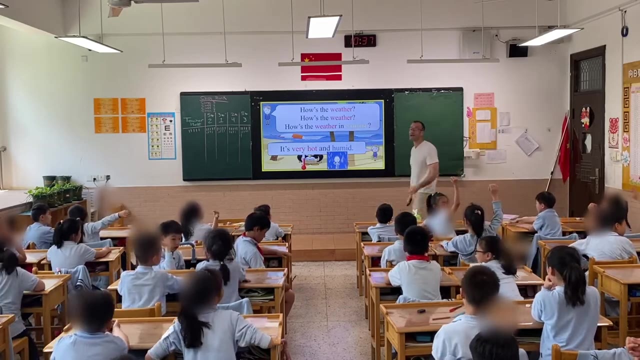 Humid, Everyone together. It's very hot and humid. Who likes the summer weather? Who likes the summer? Who likes the summer? Teacher Matt likes the summer too. I can go swimming. Good job, Any ice cream, Ice cream. 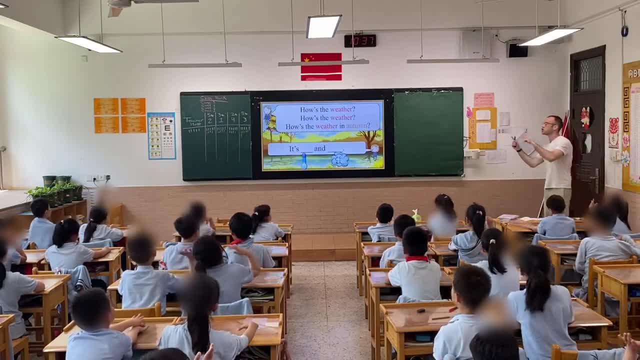 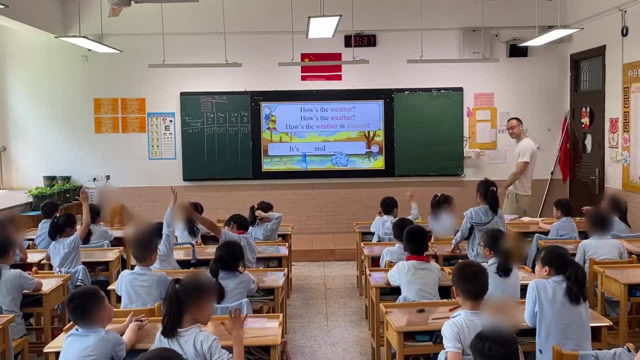 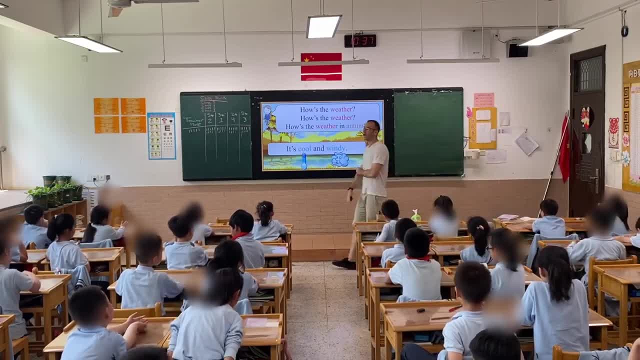 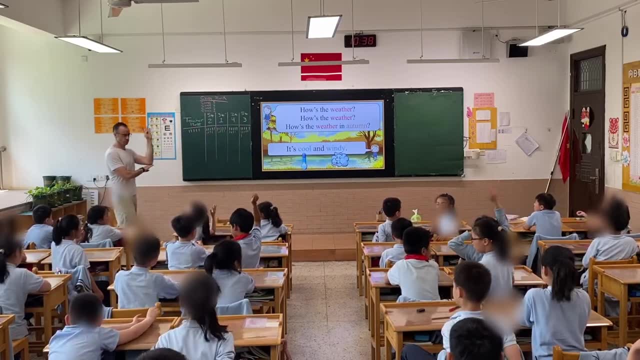 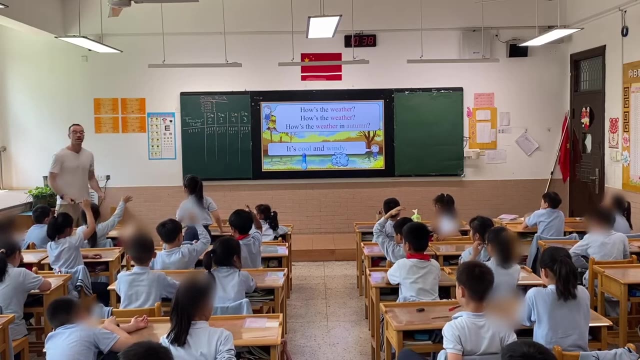 Who likes the weather in Boston? What can you do in London? What can you do in Western? What can you do in London? What can you do in the yard? Eat many fruits. Eat many fruits. yes, Play the leaves. Play the leaves. 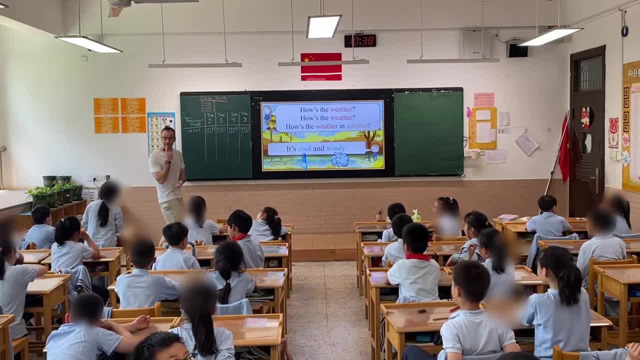 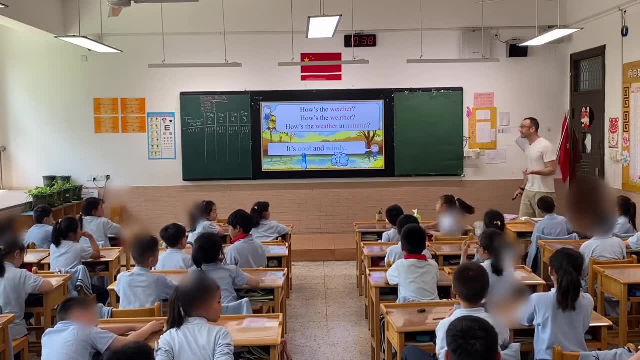 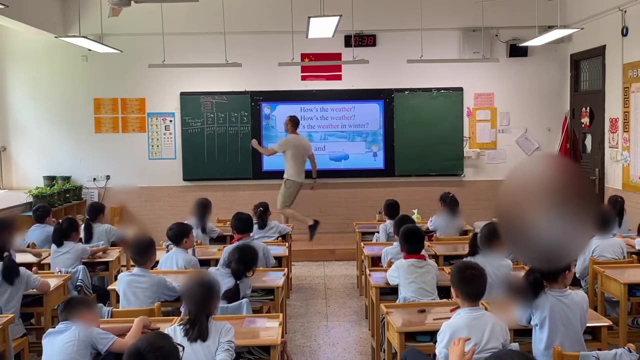 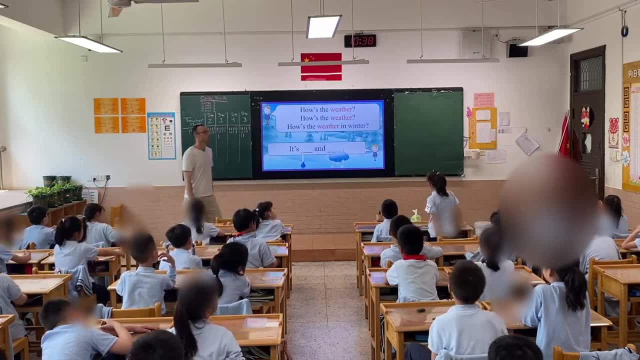 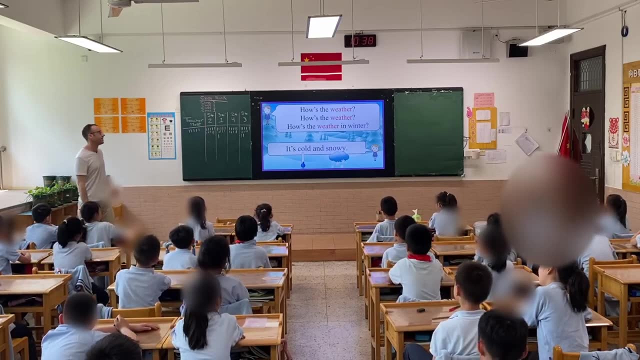 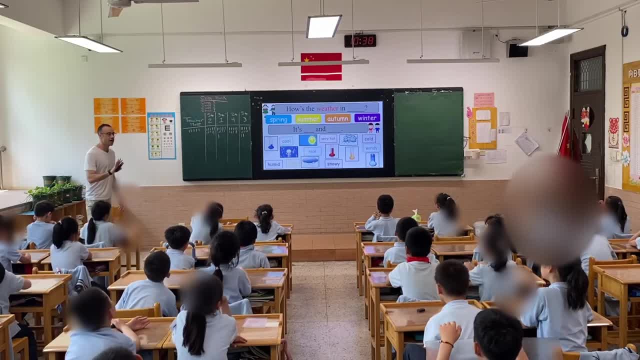 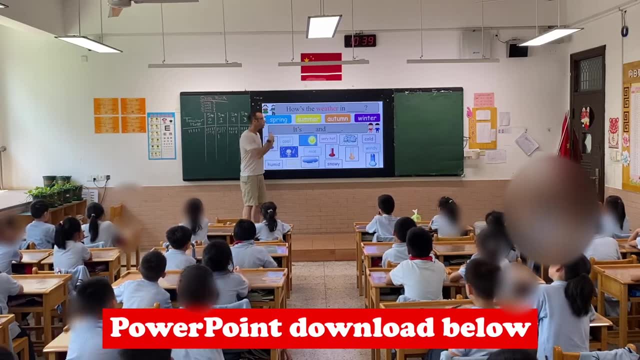 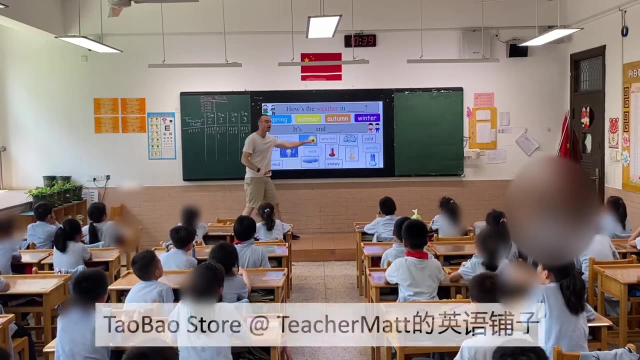 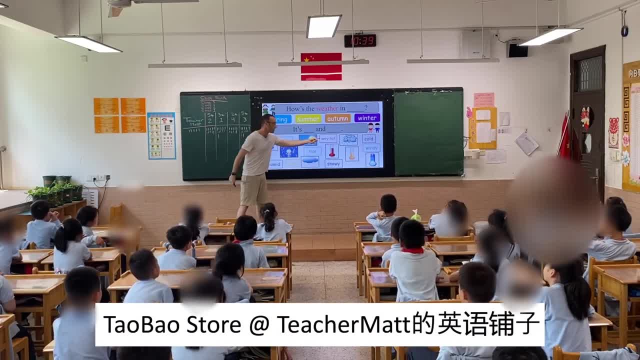 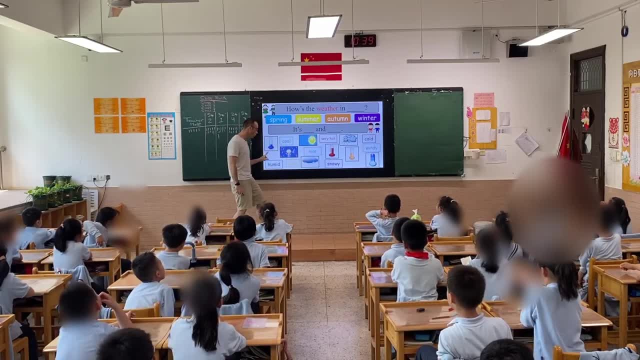 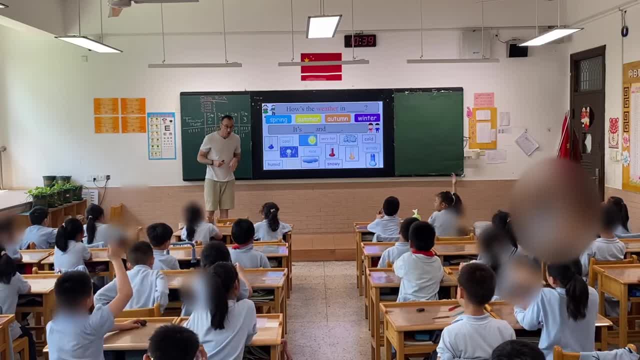 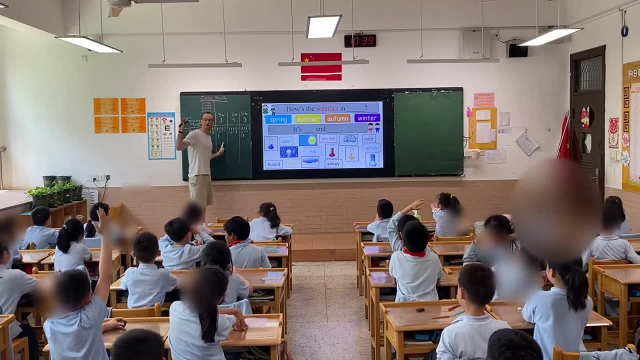 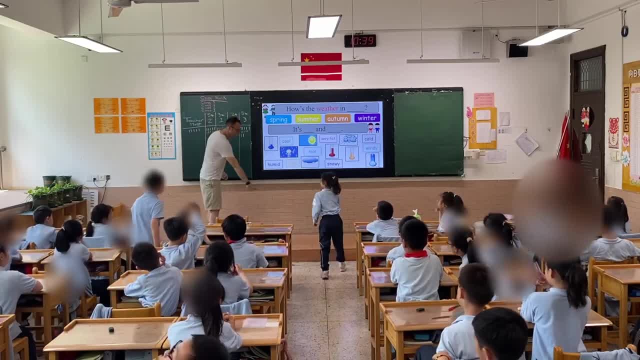 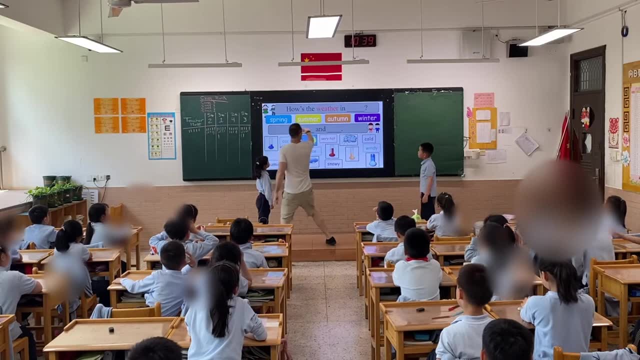 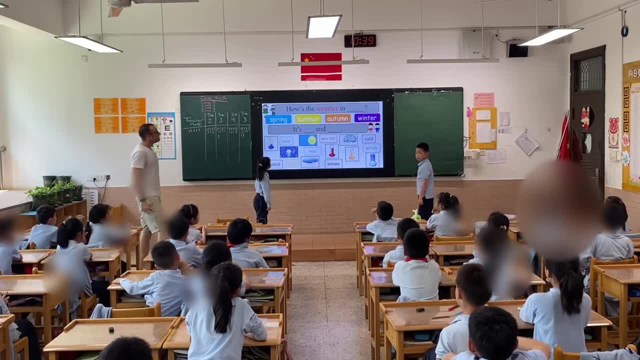 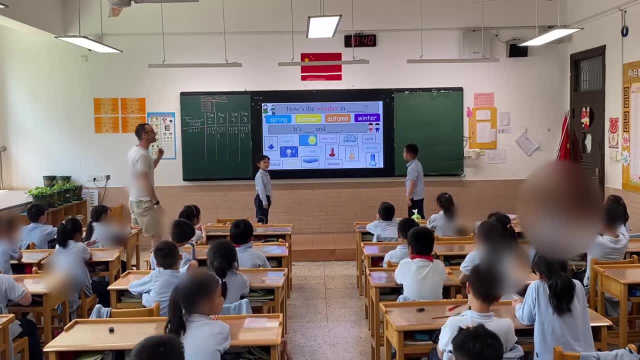 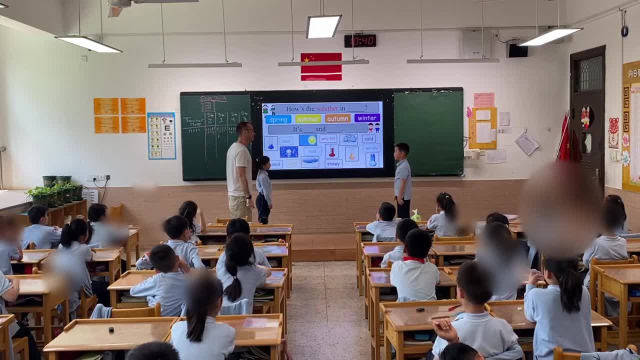 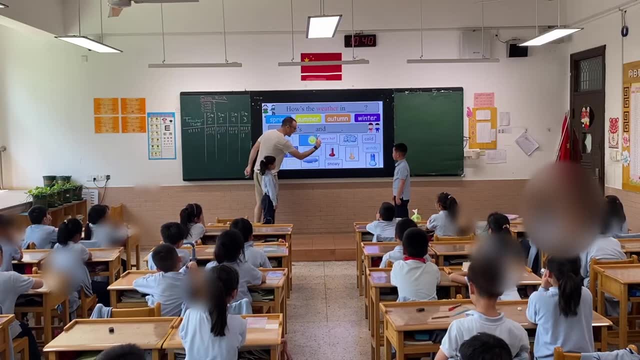 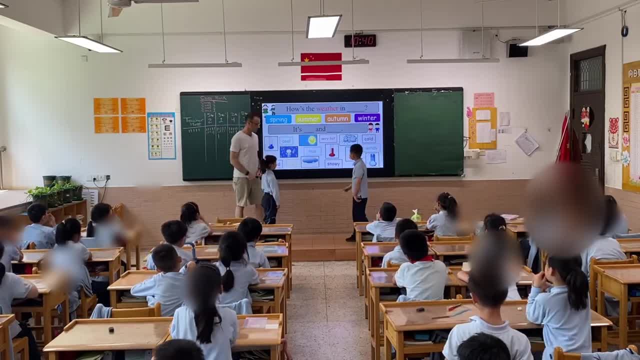 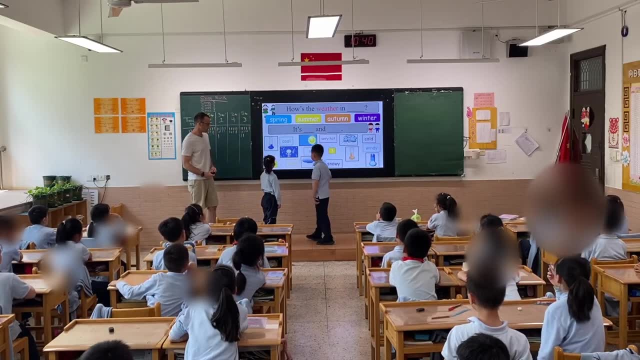 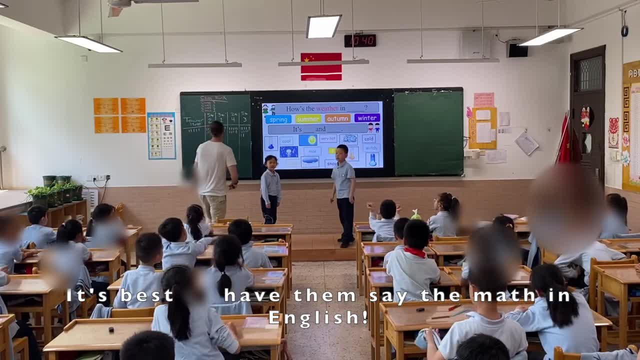 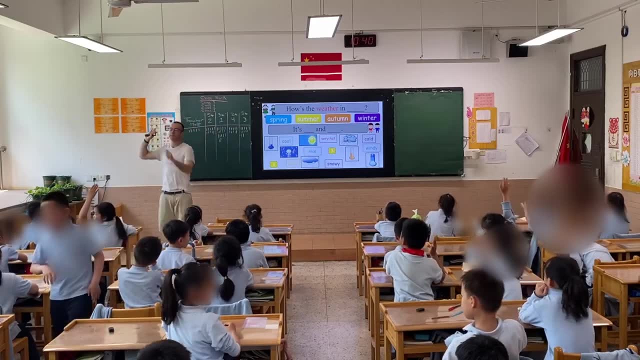 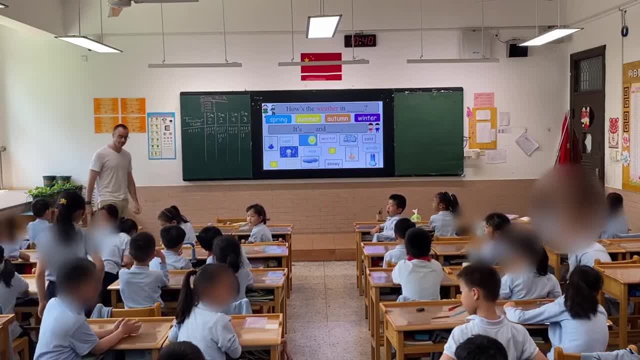 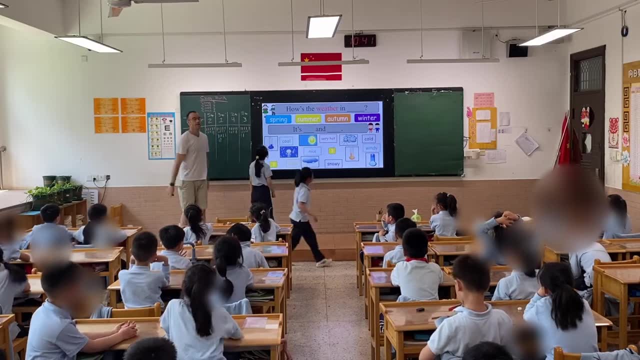 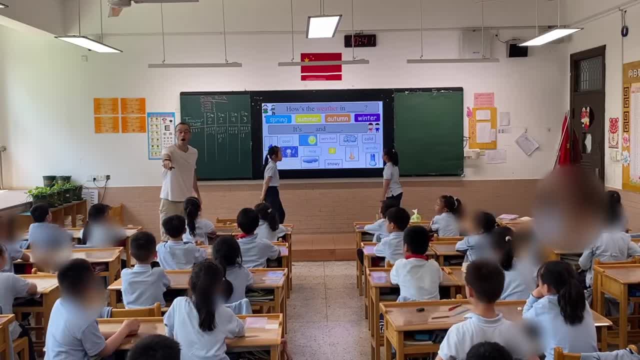 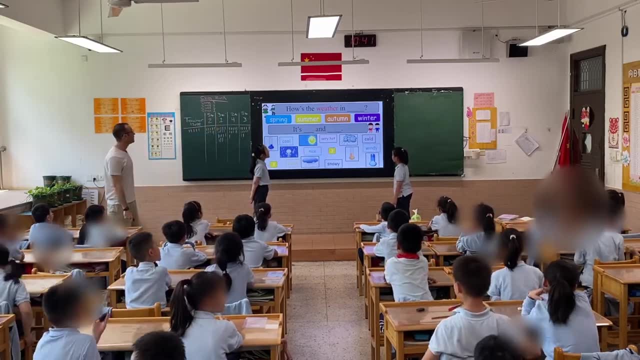 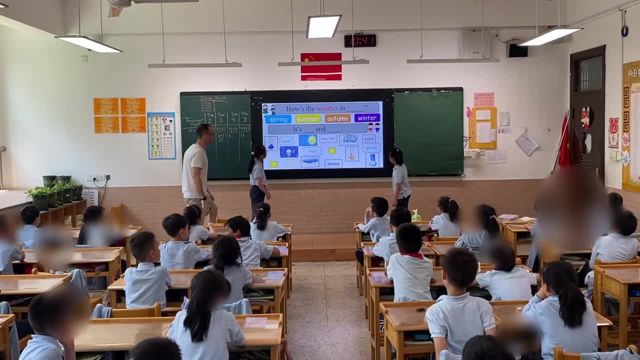 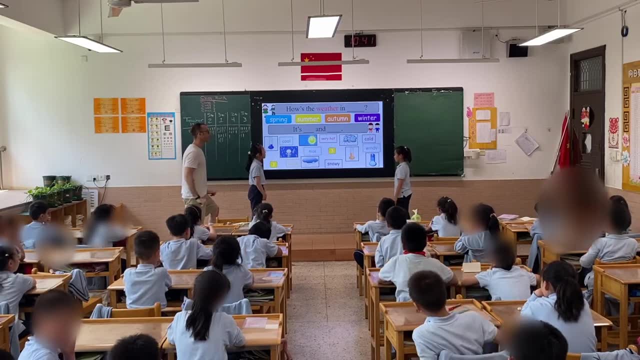 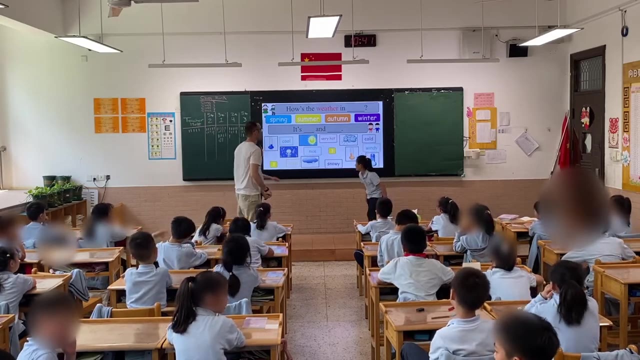 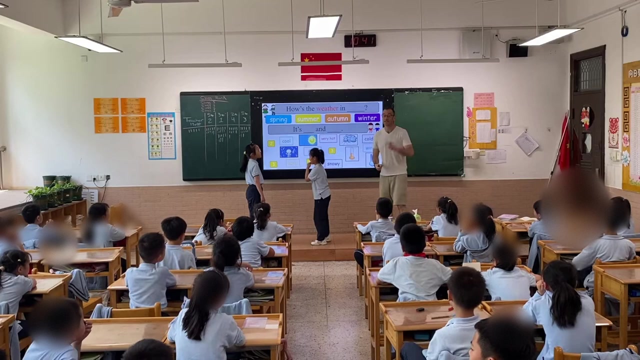 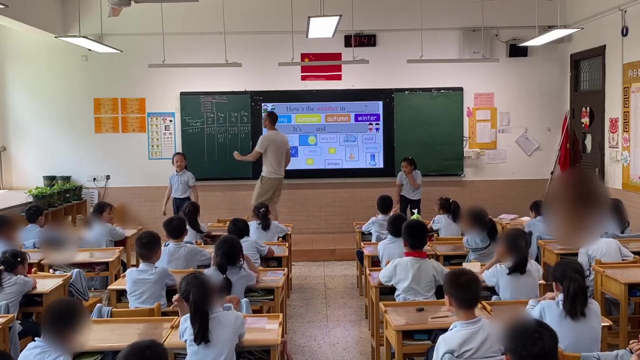 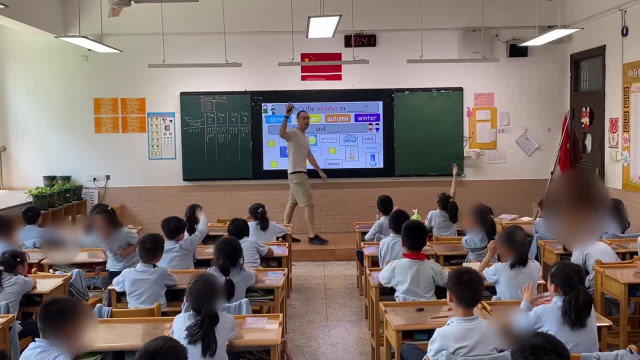 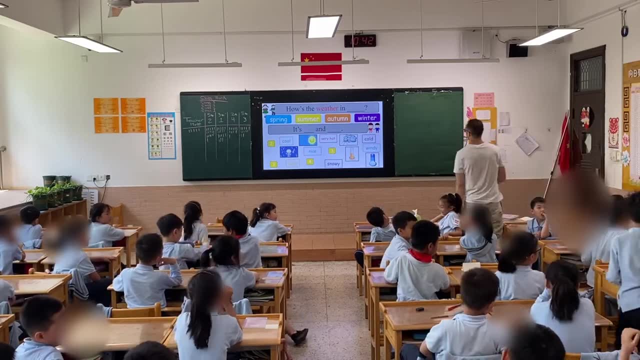 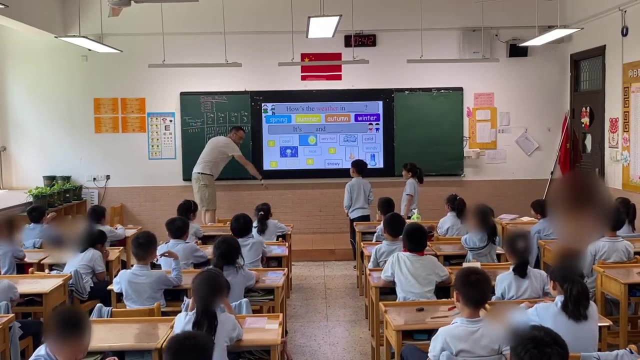 One, two, three, four, five, six, Two, three, Two, three. You're not two, three, Two, three, one, Two. Come on, So far this team is doing very well, Good job. Last four: All right, Stand And you say one. 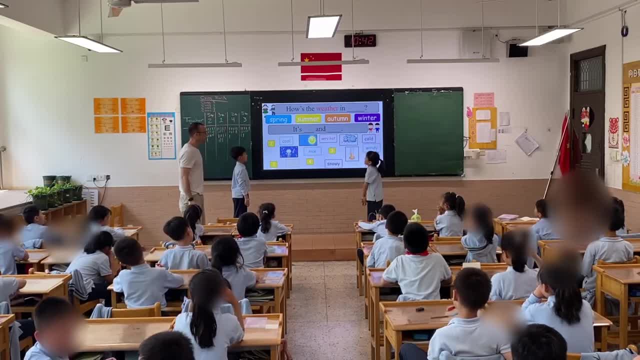 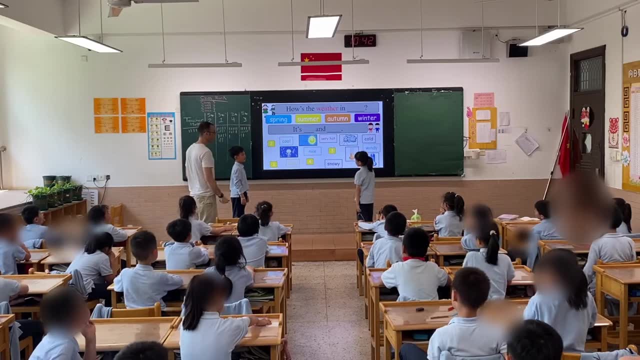 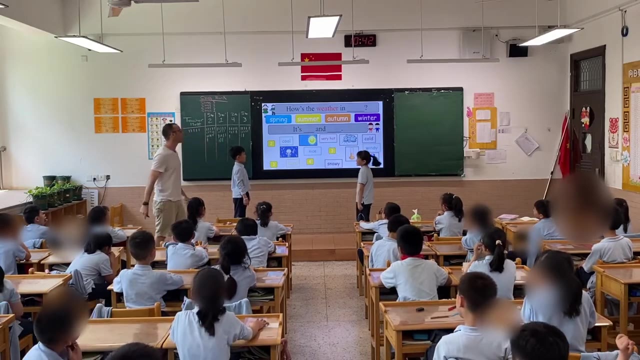 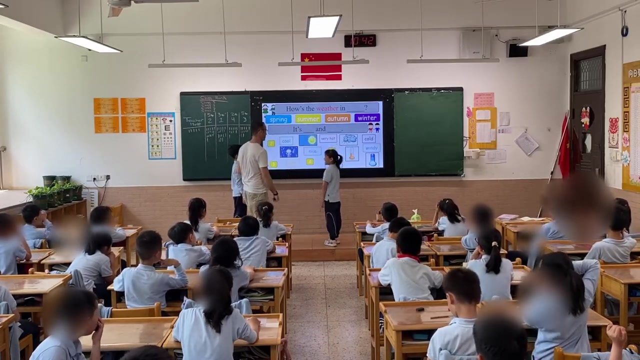 How's the weather in Boston? Everyone. How's the weather in Boston? Good, Good, Cool and windy. You can choose. Do you want this cool or do you want this cool? Do you want that windy or that Choose. Everyone say choose one. 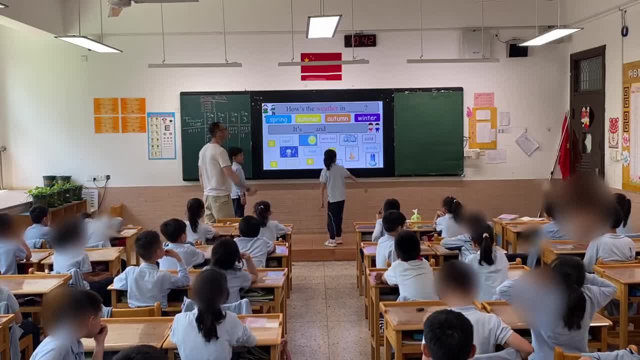 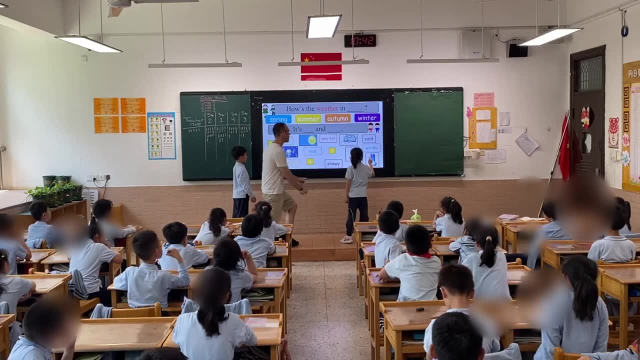 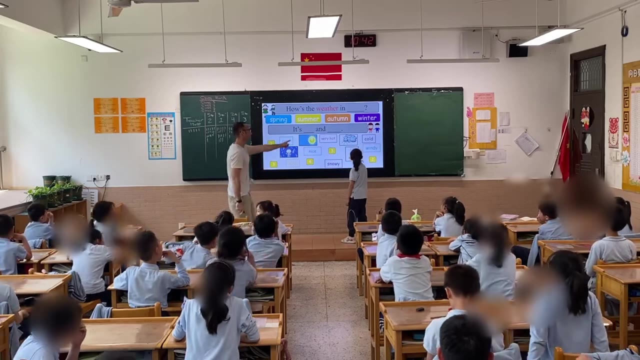 Choose one. Choose one cool and choose one windy. All right, Cool, Try again Cool. I'll try Cool And Windy. Which one? There's two windings. There's windy here and there's two here. Which one do you want? 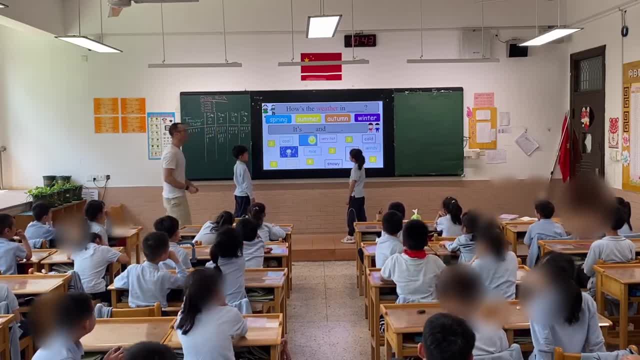 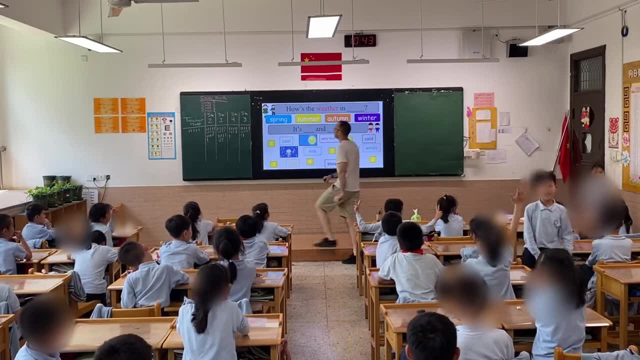 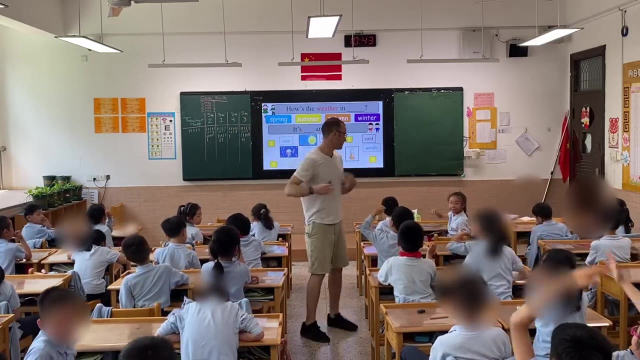 Five, four, three, two, one. All right. Two plus three equals five, All right Five. How many points for team three: One, two, three, four, five And team four: Last: two, One, two, three, two, one. 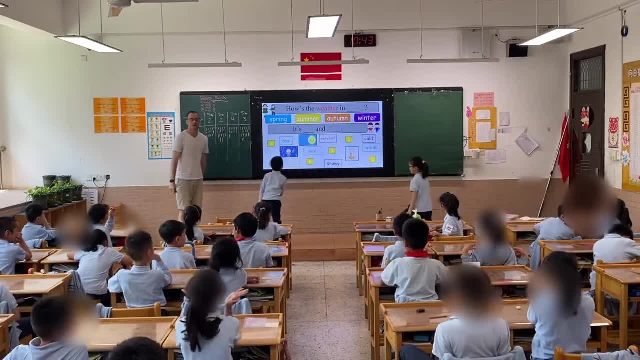 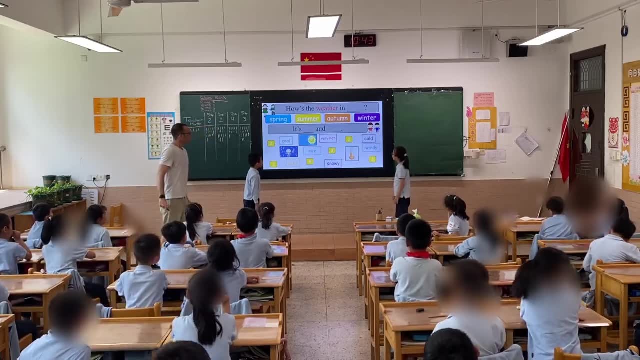 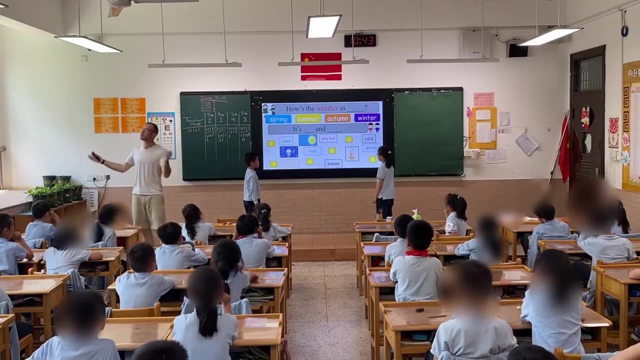 Good, All right, Good, Five, four, three, two, one Ready Go. How's the weather in the office? Good. How's the weather in Boston? Everyone, How's the weather in the office? Four, Four. 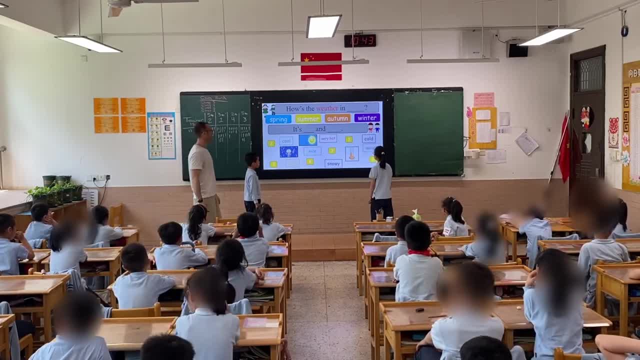 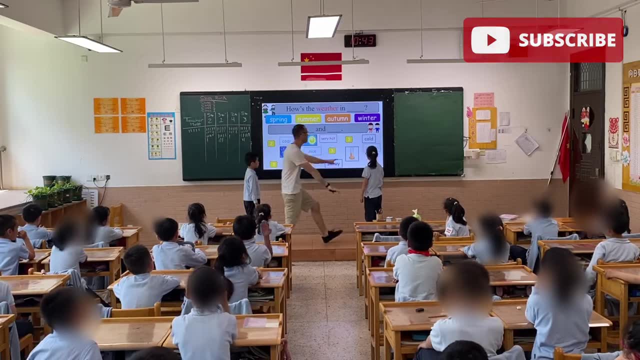 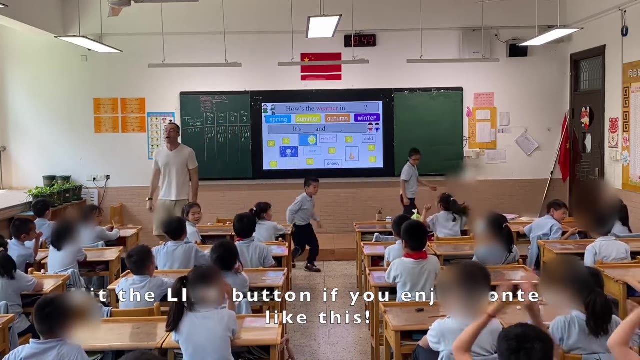 All Good, All right, There's only the words. All right, I don't know what the word is on it, but indeed, But here's something. and who is it? Four, five, four, eight, close. 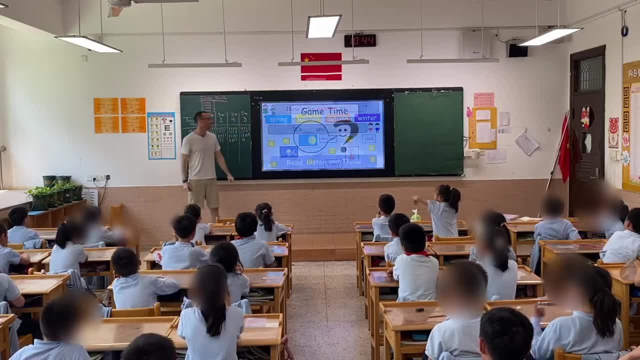 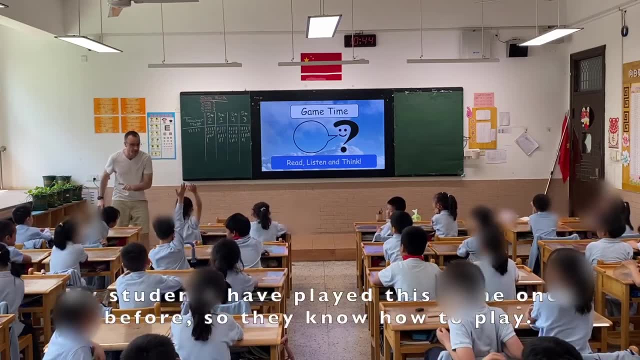 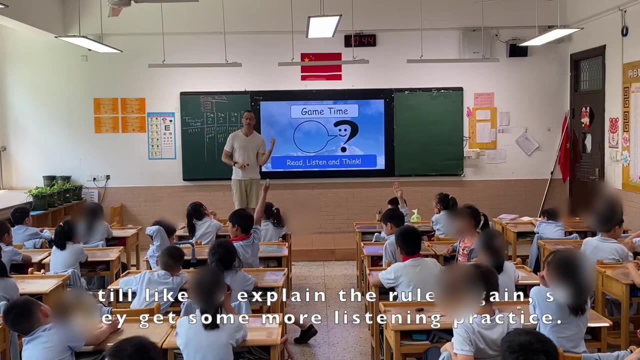 One, two, three, four, five, six, seven, eight. Good job, right, listen to me. So that's like I need one student from each team to come here and stand here. These four students can't look at the screen. 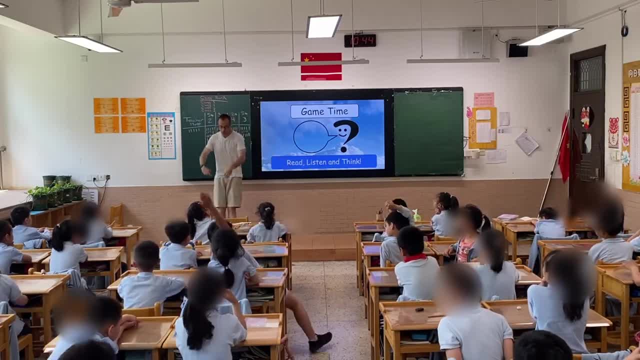 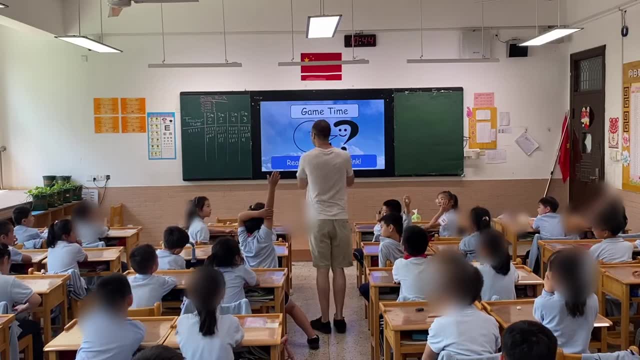 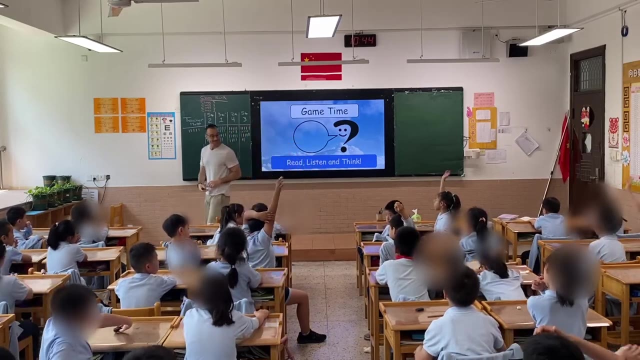 This is the green. Listen at the same thing. One student here, here, here and here looking this way, One student to read, And these four students must listen and say which season. Okay, All right, Bring on four good students. 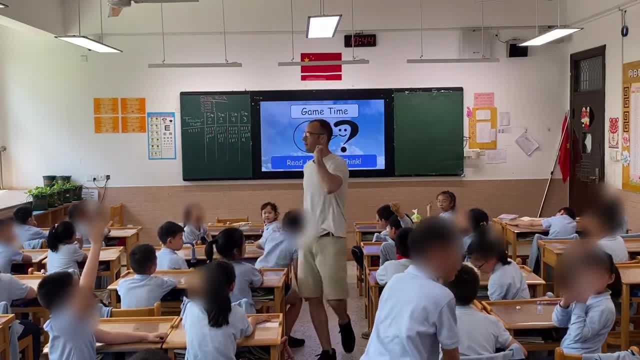 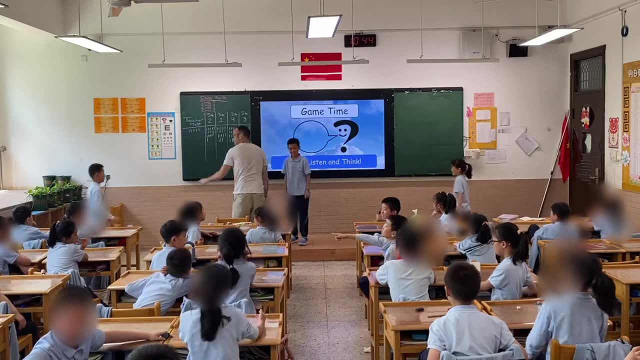 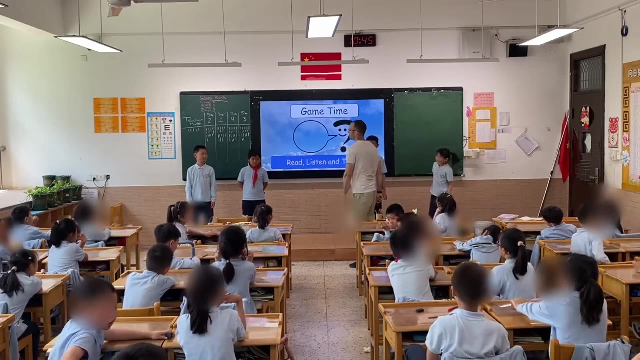 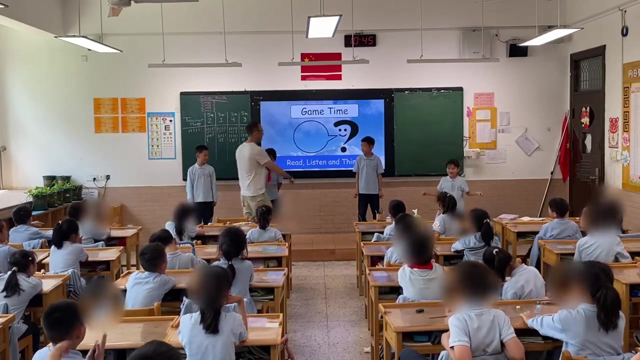 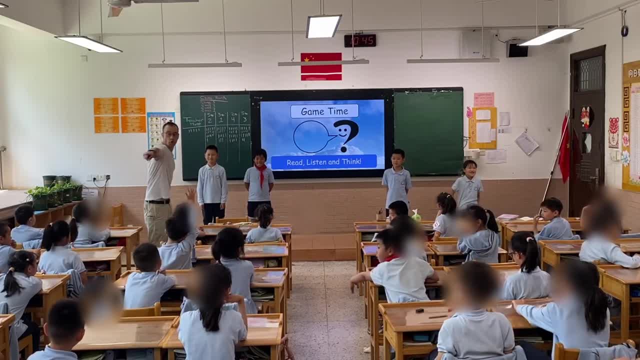 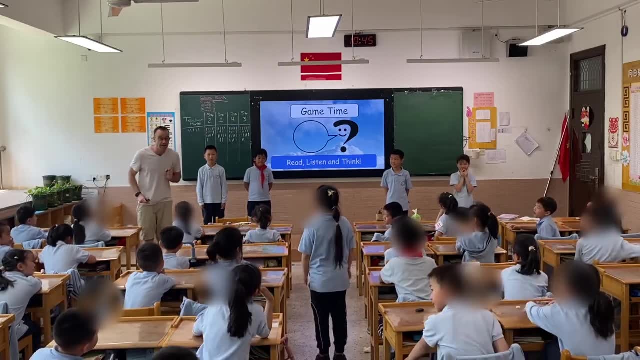 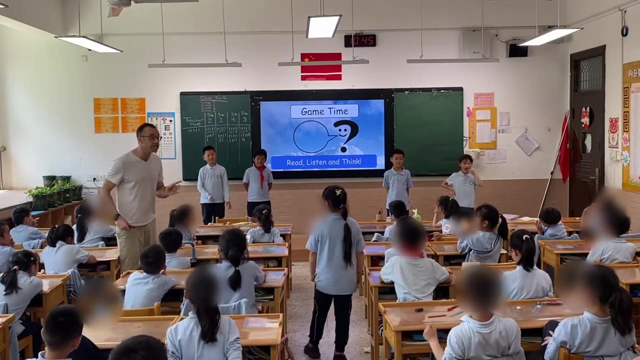 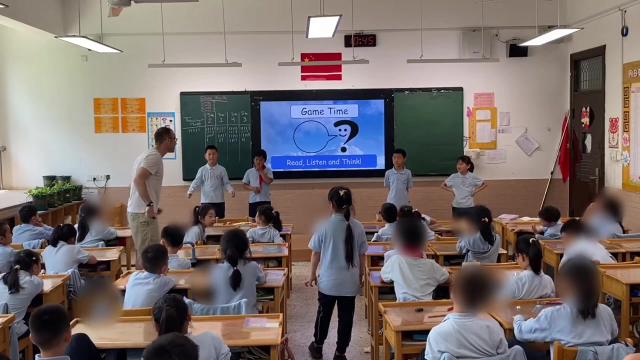 All right me, stand here. Okay, I'm walking here instead of them. Everyone be quiet. If you say the answer, if you say the answer, your team will lose points. Okay, Okay, Are you ready? Let's do it nicely. 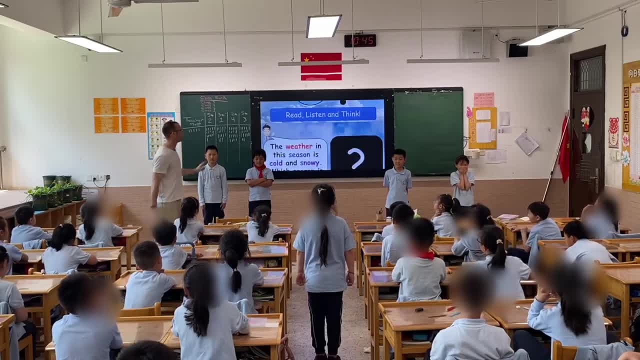 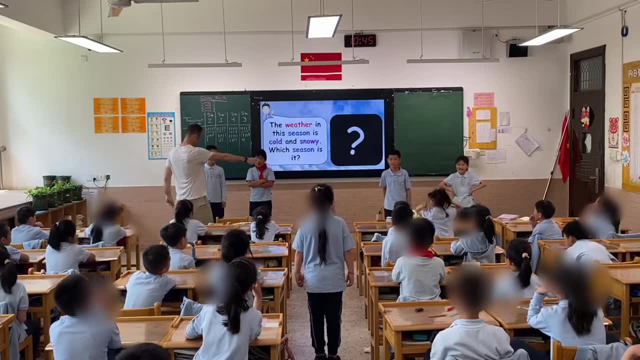 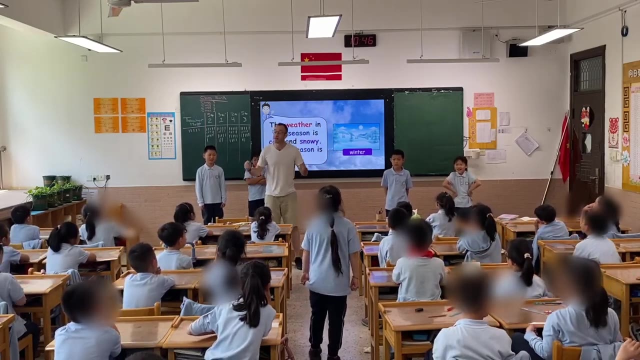 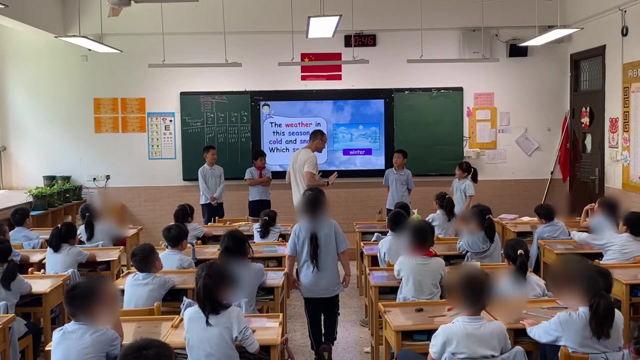 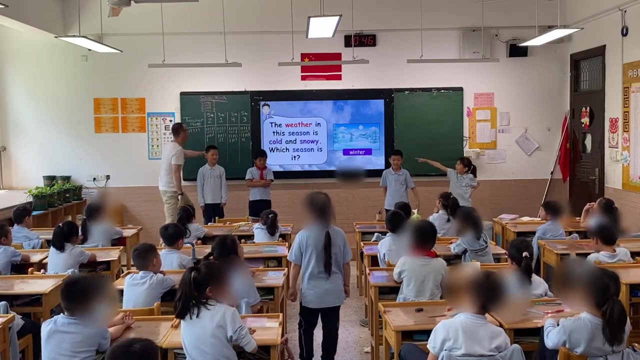 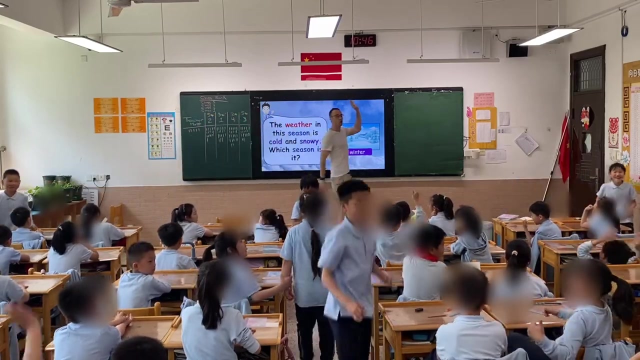 and snowing. Which team are you? Which team? Four, Team four, One, two, three points. Go sit down, Go sit down. Good job, Andy, Go sit down, Go sit down. Excellent, One, one, one one. 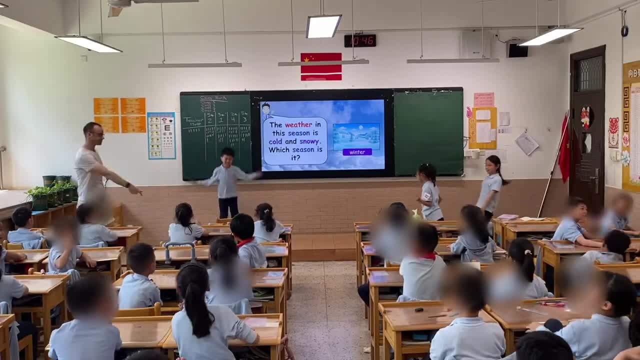 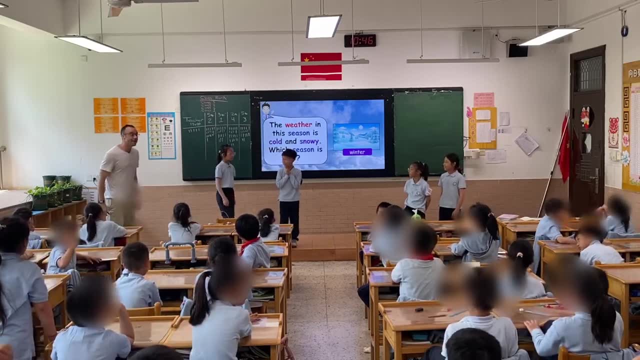 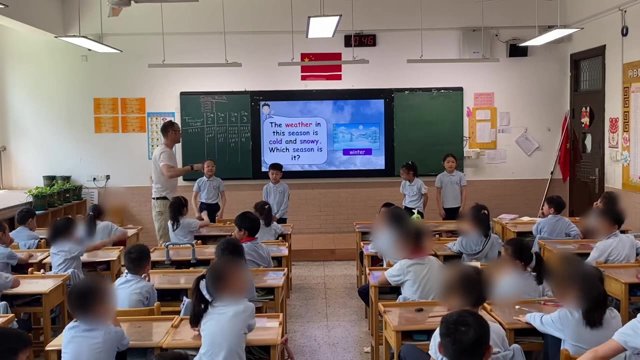 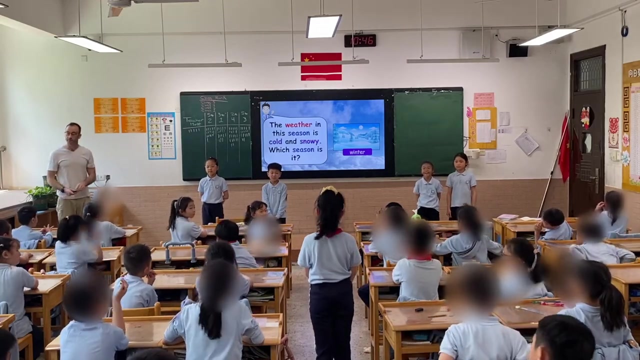 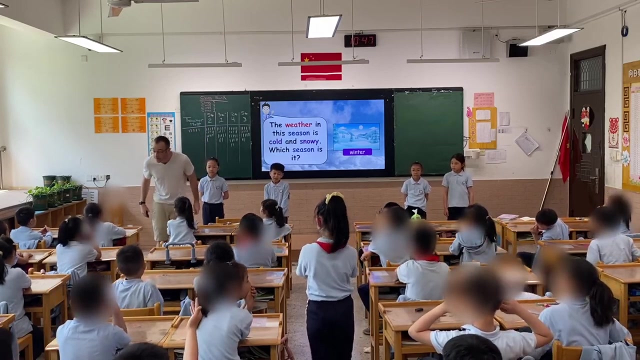 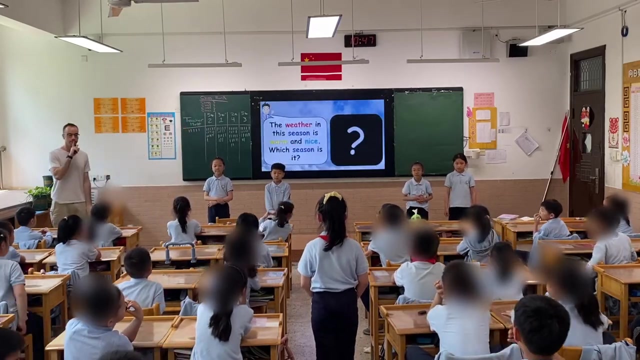 Who would like to read? Alright, come on, Stand here. Five, four, three, two, one. Are you ready? Ladies, be quiet. No action. Okay, sit nicely. Are you ready? The weather in this building is one of mine. 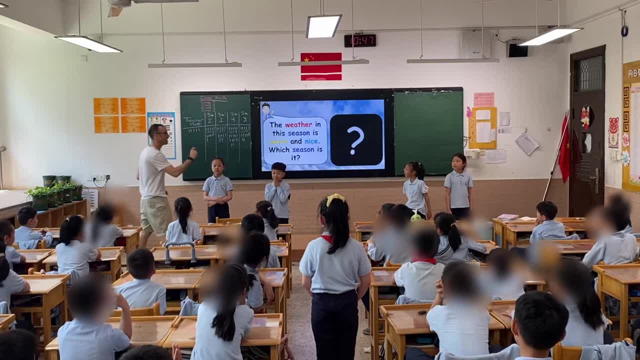 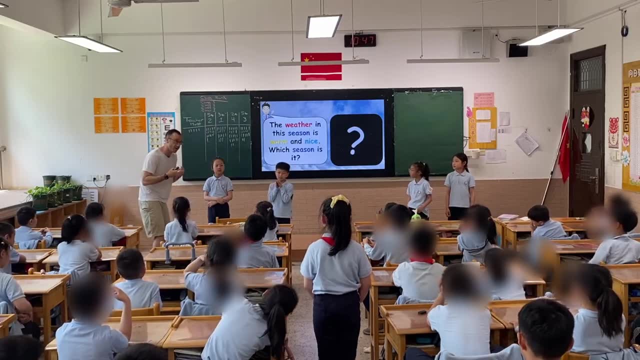 Alright, I think it was a tie Very, very close here, Very, very close. I'll give points to you and points to you Very, very, very close. Alright, everyone ask how's the weather in spring? 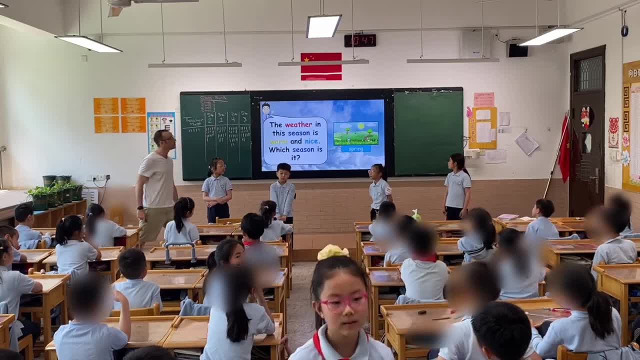 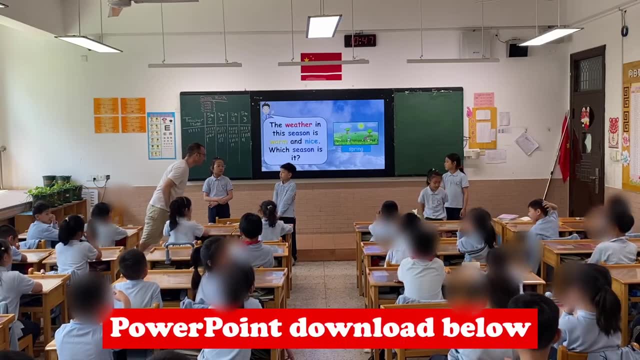 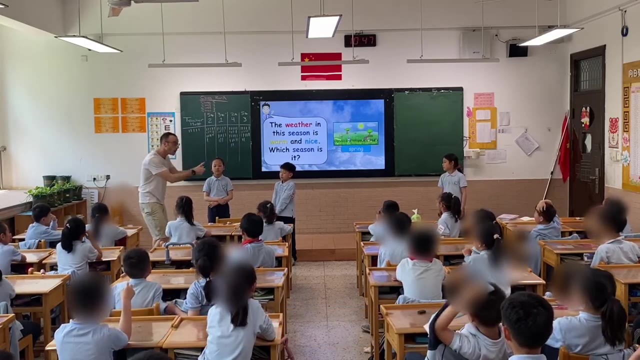 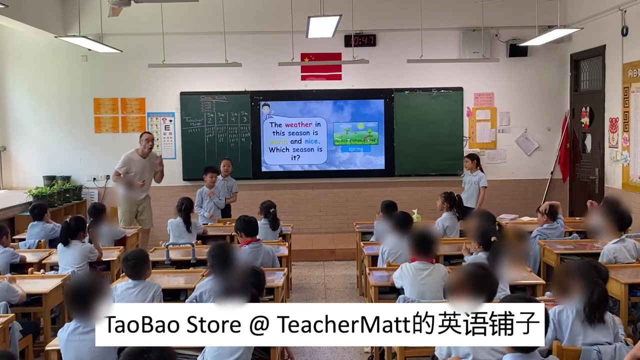 How's the weather in spring? Spring is warm and it's nice Good. How's the weather in spring? Good, Warm and nice. Everyone, spring is warm and nice. Good, Ada, which team are you Four? 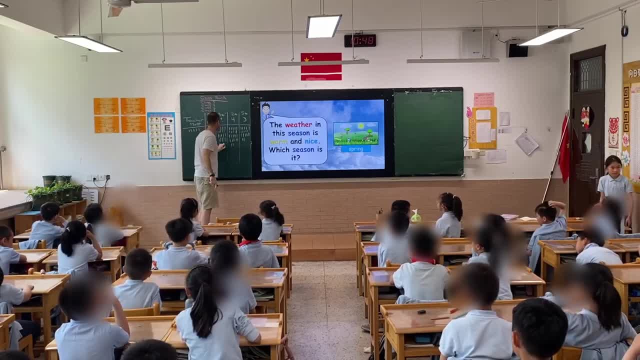 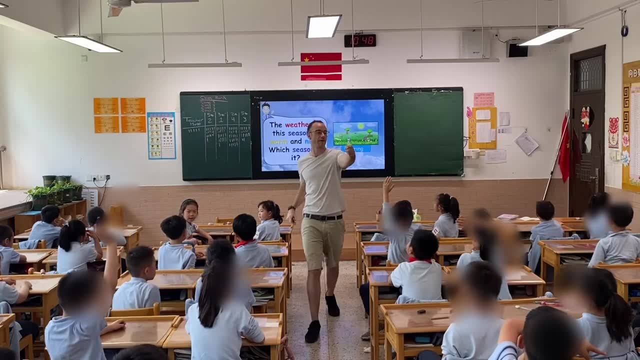 Four. And which team are you? One One, two, three. One, two, three. Who would like to try? Who would like to try? Who would like to try? Alright, Katherine, Come on, Come on up. 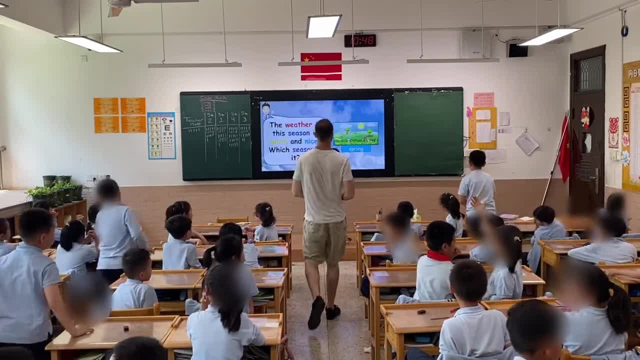 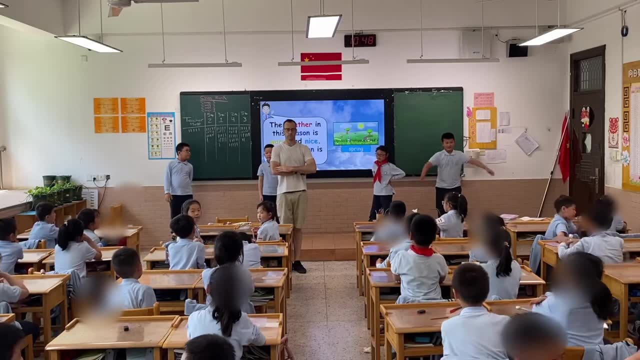 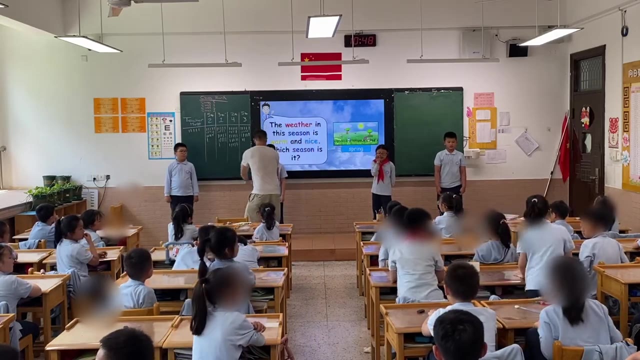 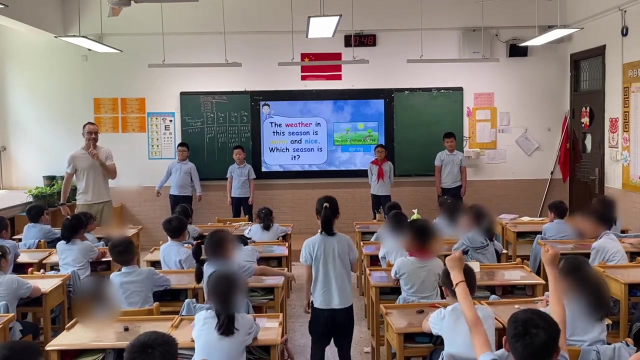 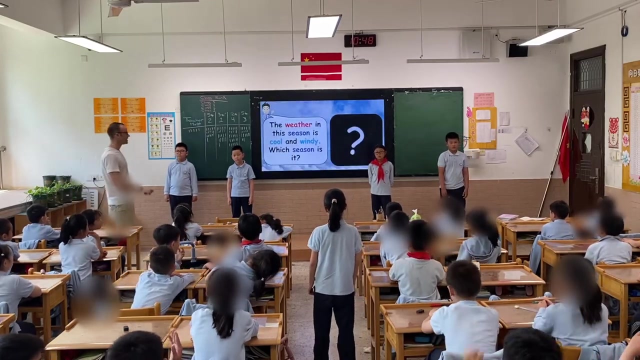 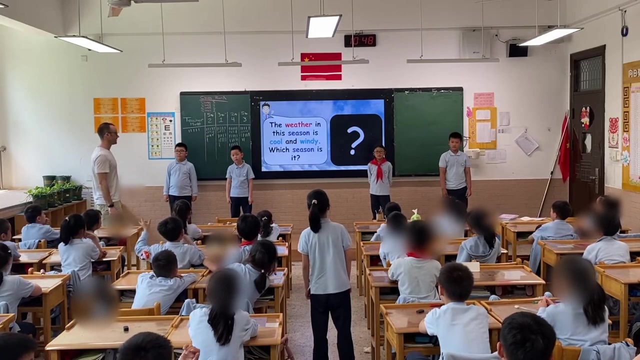 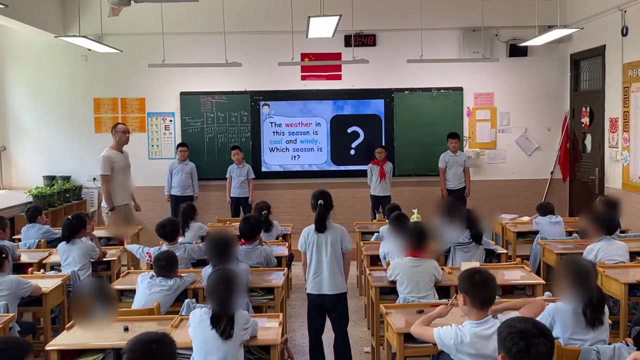 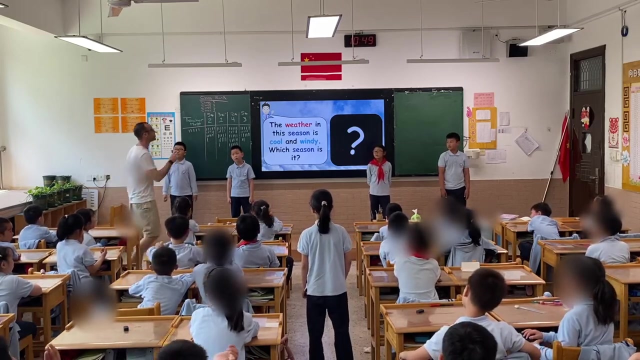 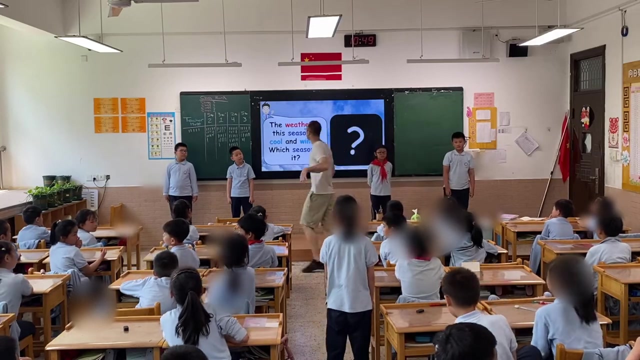 Katherine, stand here. Five four, three, two one. Which team is talking? Who would like to read? Five four, three, two one. Be quiet, Are you ready? 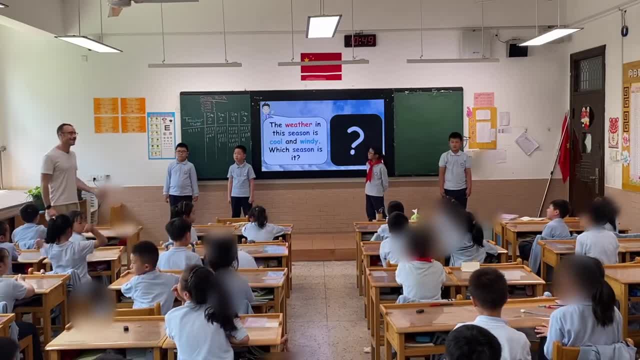 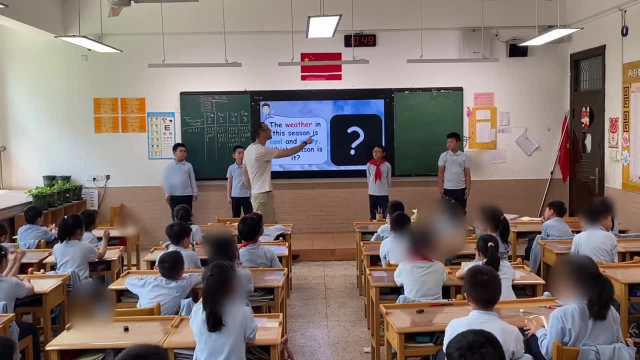 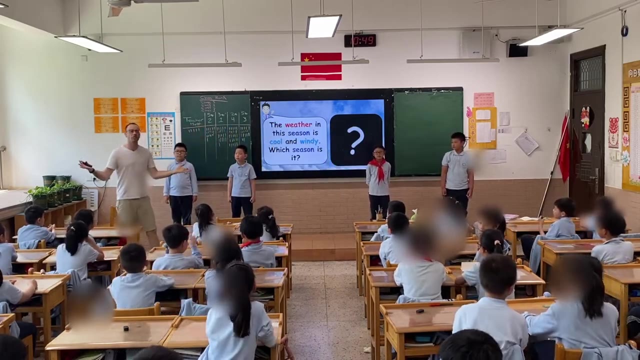 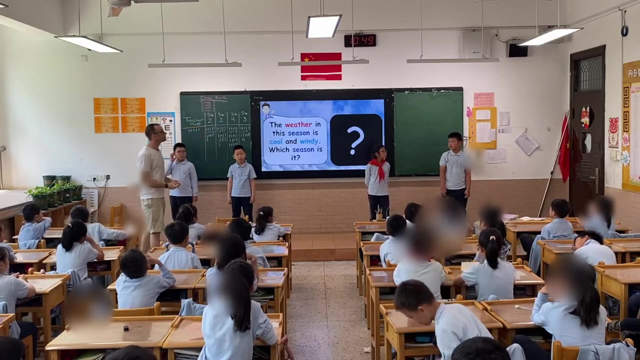 Who can we meet? Which season is it? It is Autumn, Everyone. Autumn, Autumn, Autumn. He's asking: how's the weather in Autumn? Ask him: How's the weather in Autumn? How is it? It's sunny. 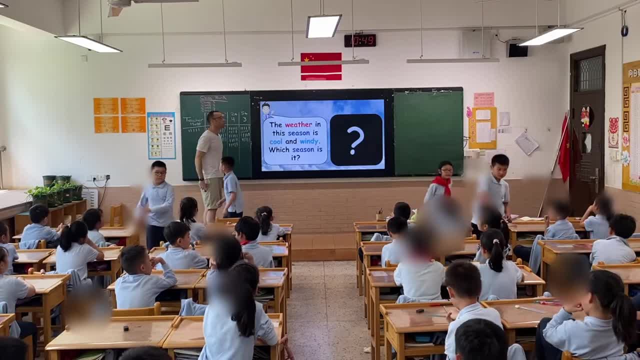 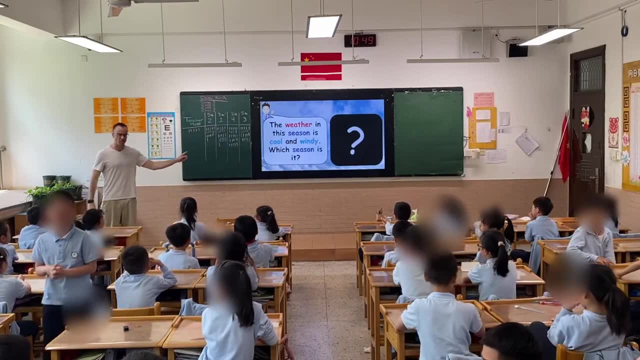 That's right. Good job, Post it down. Three points to the team Three. Good job, High, high, high. Post it down. What's the last one? What do you think the last one is? What's next? 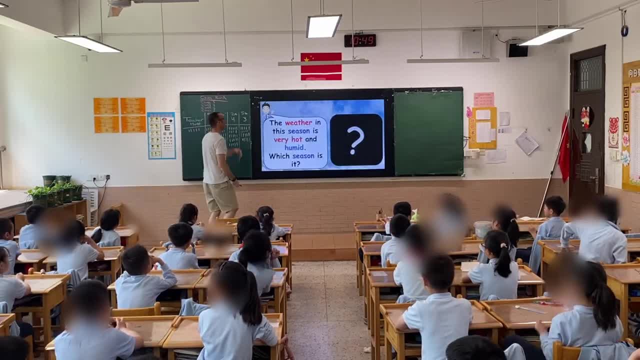 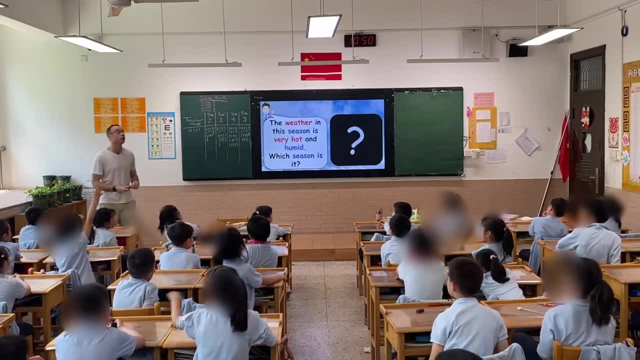 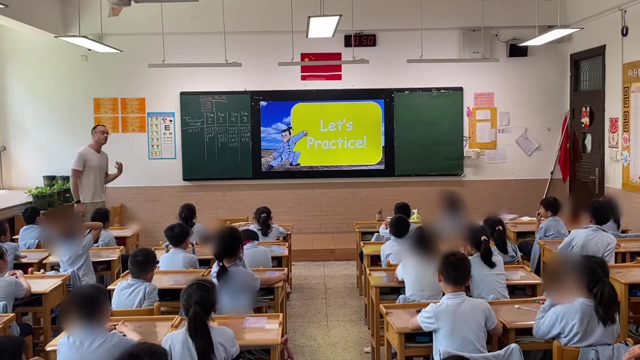 Summer, Good, Everyone read it together. Everyone read it together. The weather in this season is better than in June. Which season is it Summer? All right, Good job, Let's practice more Everyone. let's practice, Let's practice. 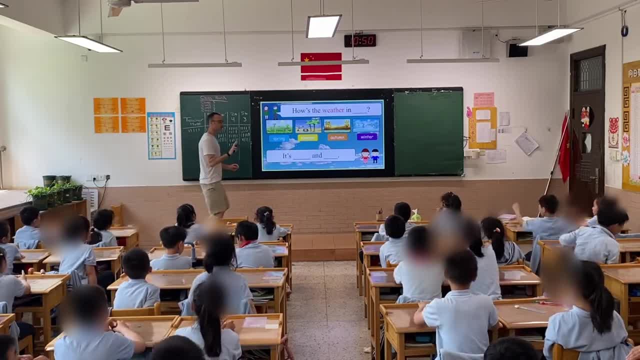 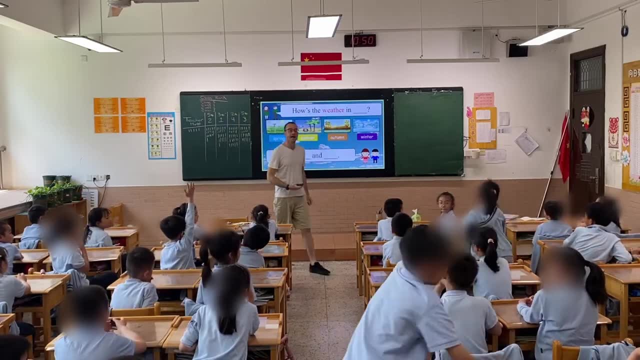 All right, Take a look. Take a look. Here's how it works. Two students Show as an example. All right, One and two. Actually, we can do it the first time. It will happen. Don't need the example. 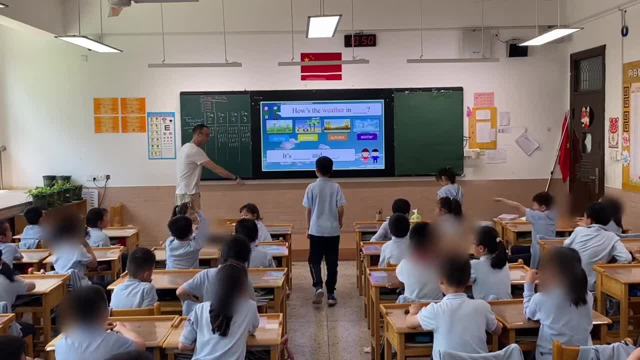 Very easy. You stand here, You stand there, All right. You say: how's the weather in June? How's the weather in June? How's the weather in summer? Good, How's the weather in summer When it happens? 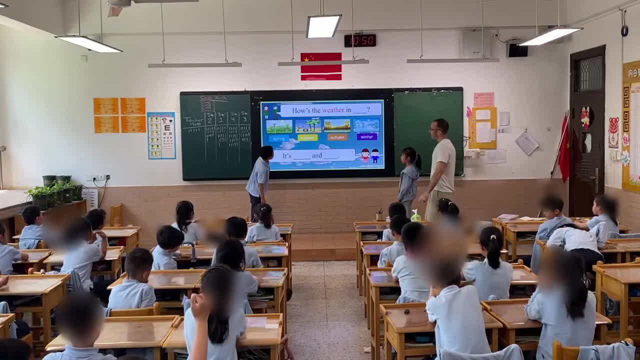 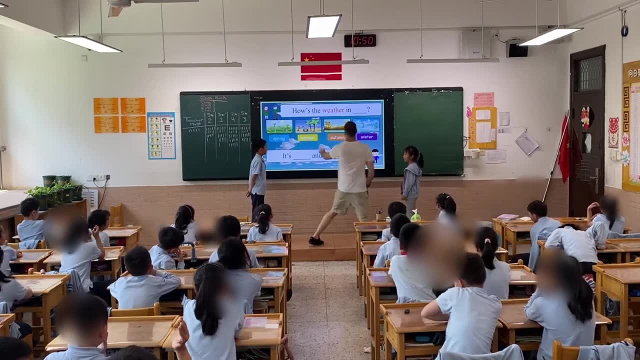 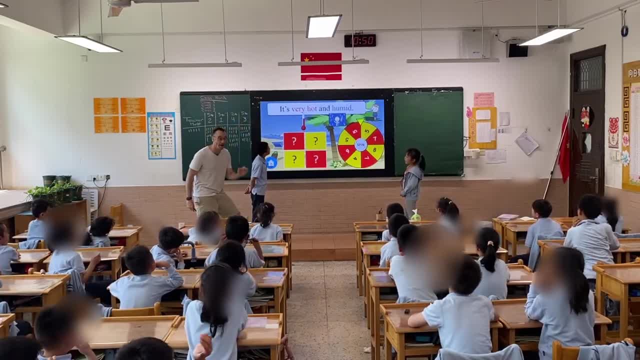 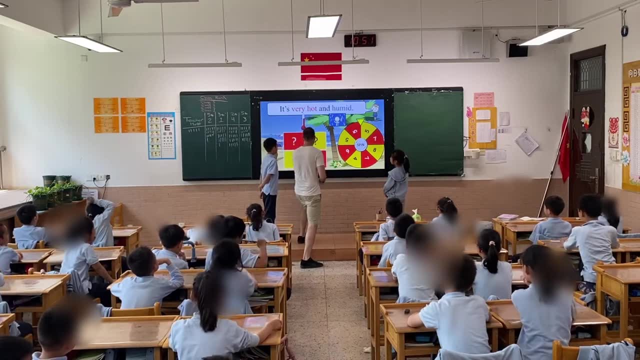 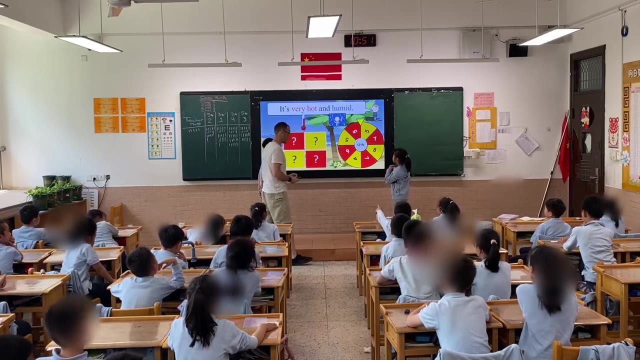 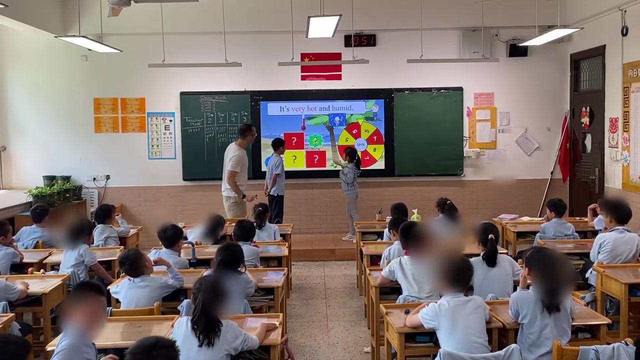 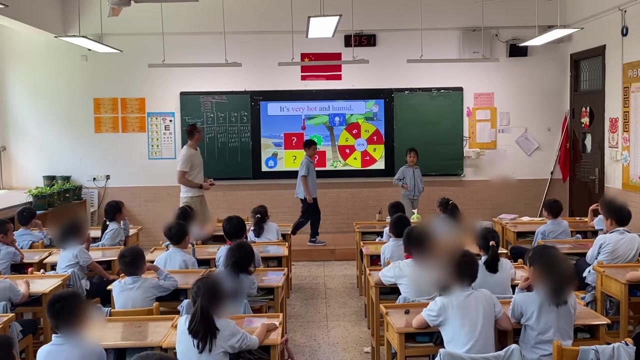 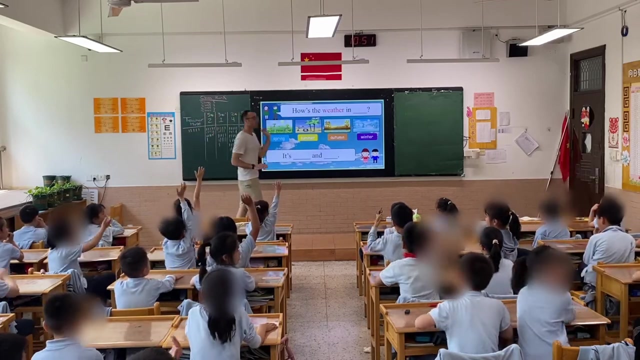 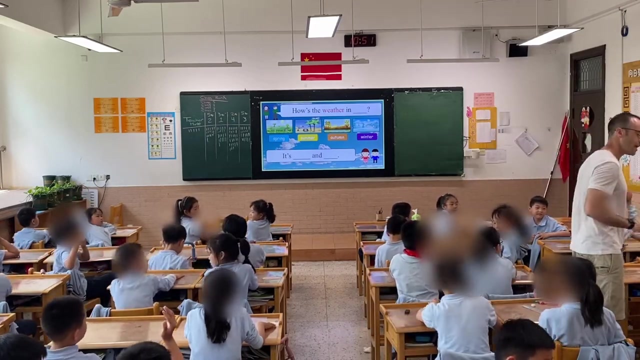 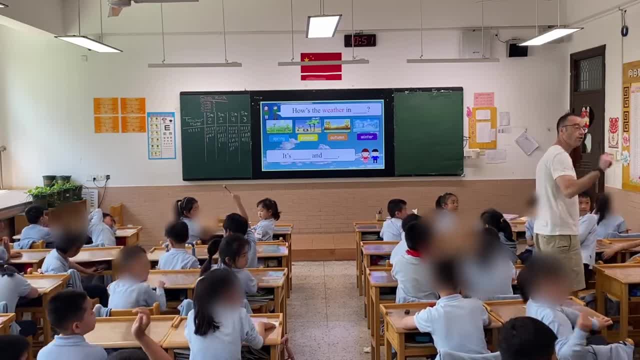 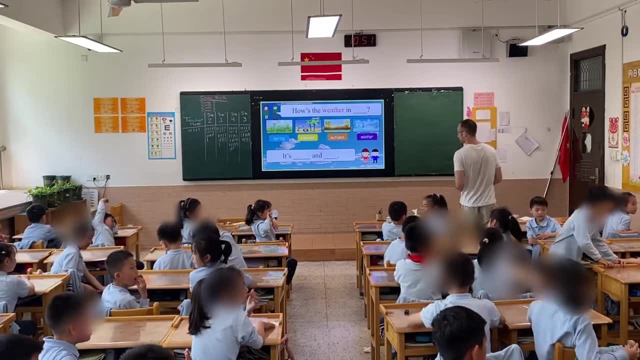 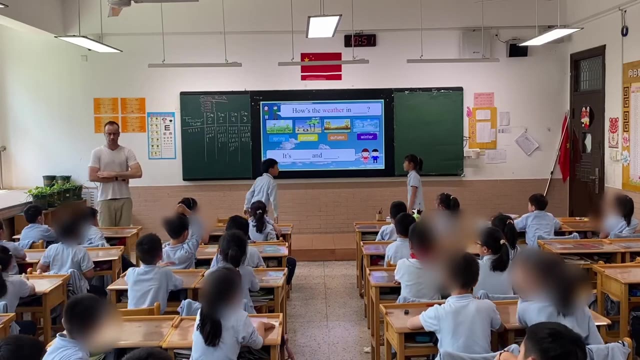 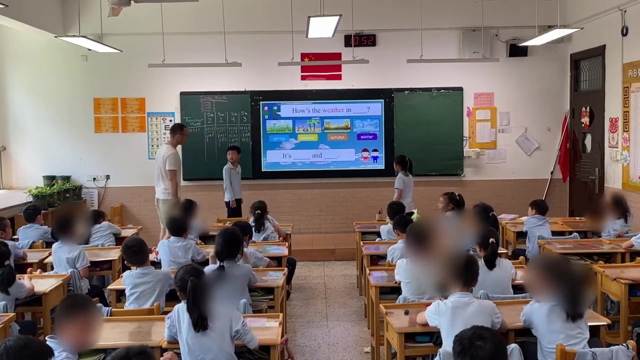 Who did not play this game? Who did not play this game? Come on, Come on. 5,, 4,, 3,, 2, 1.. Sit back and sleep, Alright. ask, choose a season. How's the weather in? Choose one. Say, how's the weather in? 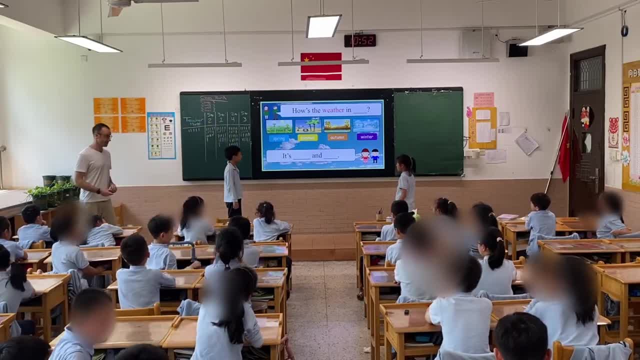 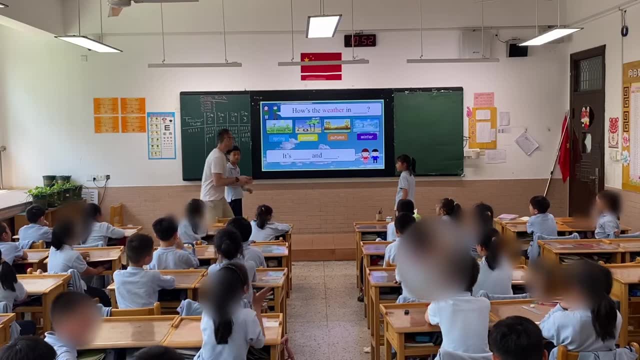 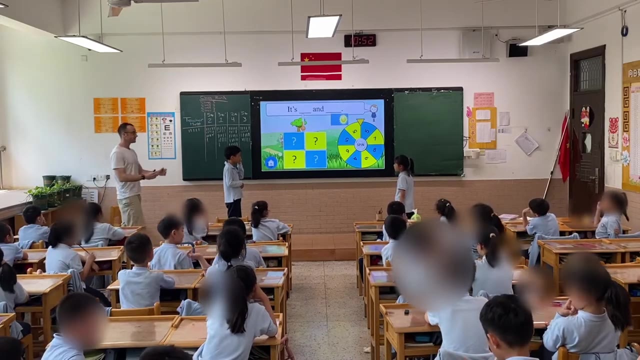 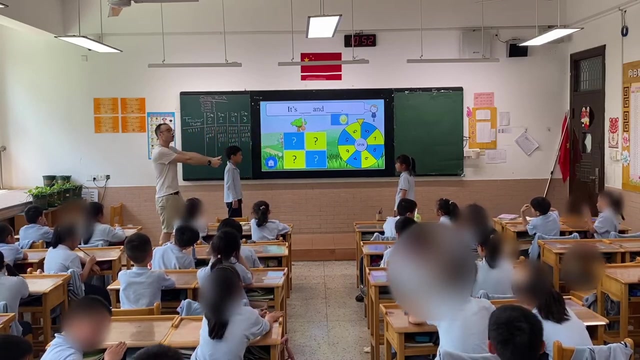 Good, How's the weather in Spring? Spring is cool, It's. Let's get some help. Let's get some help. Take a look How's the weather in spring. It's Who can help her. It's warm and good. 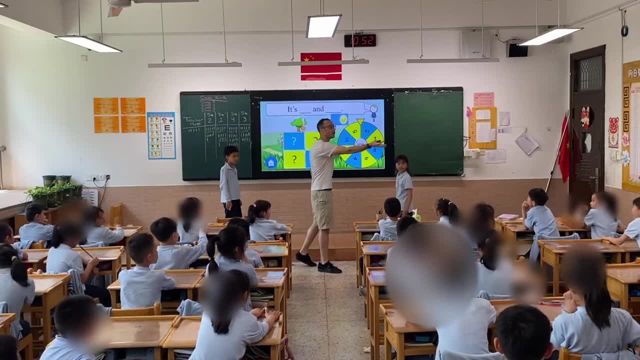 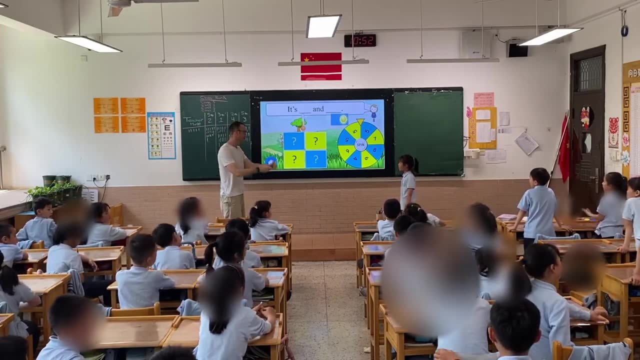 How about Team 3?? Stand up, Team 3, stand up and help her Say: everyone together on Team 3.. It's warm and nice. Good, Warm and nice. Okay, Alright, you choose. You can choose any box or spin the wheels. 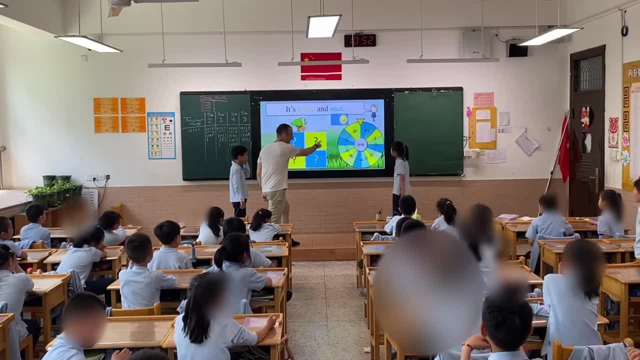 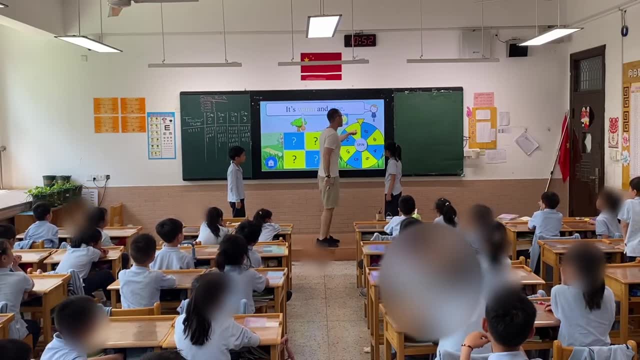 Spin the wheels, Alright, push it And push it again, Push it again. 1,, 2,, 3,, 4,, 5,, 6,, 7, 8.. It is 7.. It's on this side, 7. Good job. 1,, 2,, 3,, 4,, 5,, 6,, 7.. 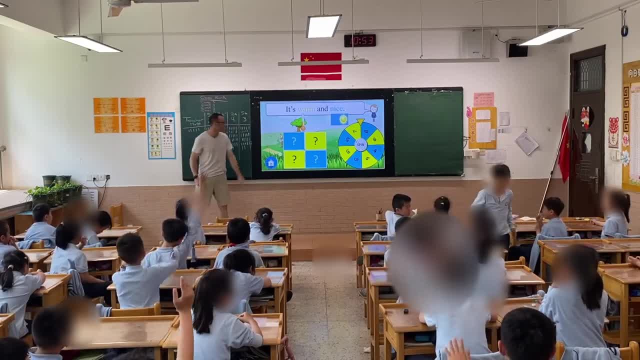 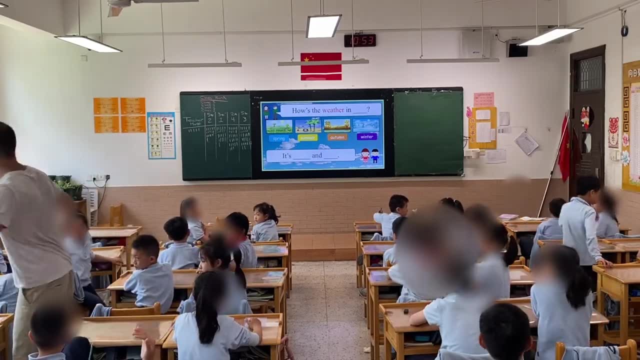 10. Alright, Team 2. Team 2. Team 2.. Alright Leo, 1, 2,, 3,, 4,, 5,, 6,, 7, 8.. That's warm. 1, 2.. 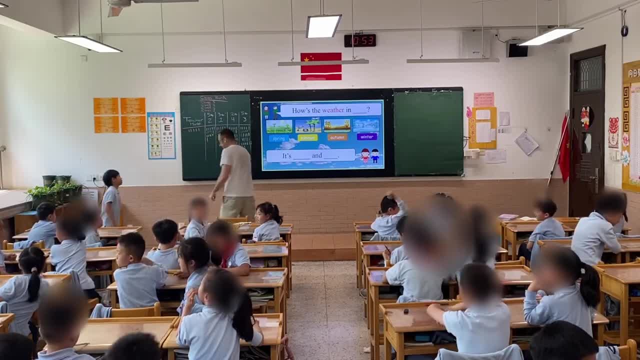 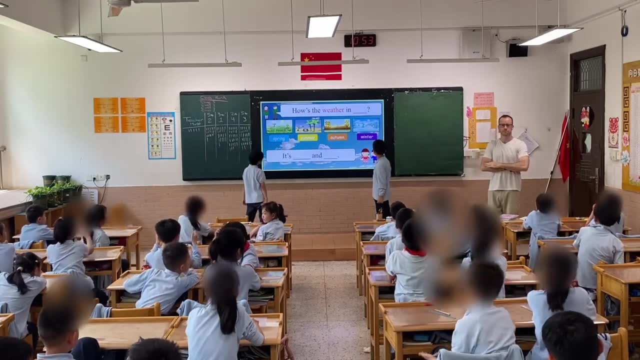 Yeah, yeah, I've got to sit 5,, 4,, 3,, 2,, 1.. 1, 2.. Leo say: Mom, Mom, Mom, Mom, Dad, Mom, Mom Mom. 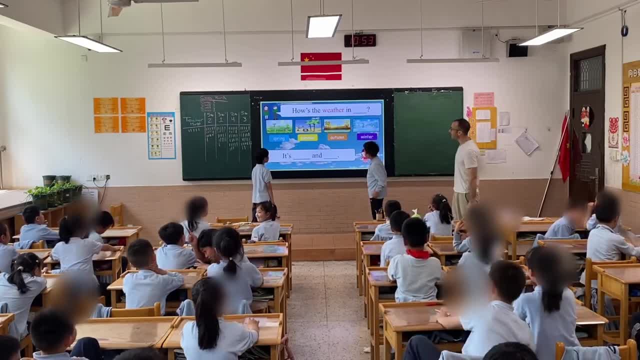 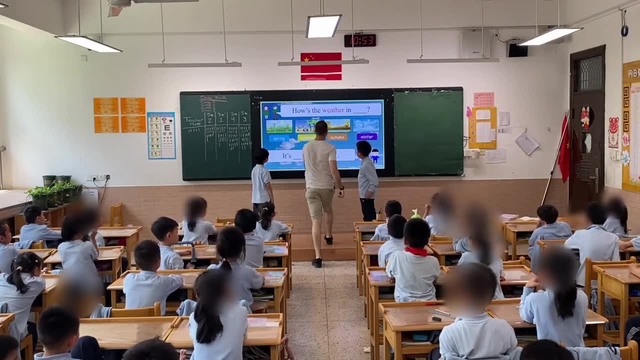 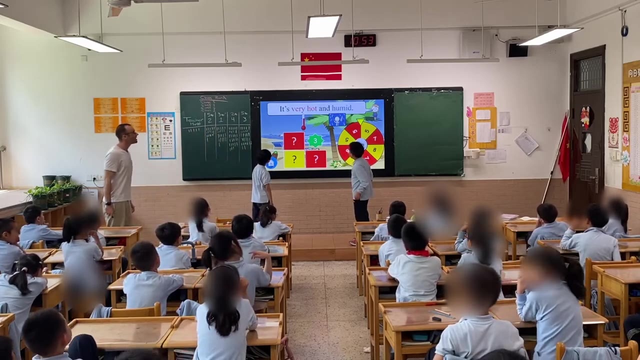 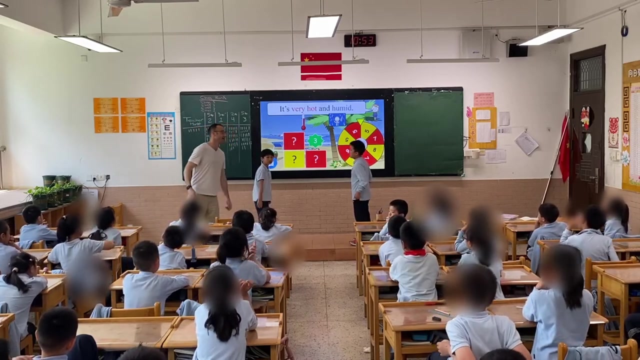 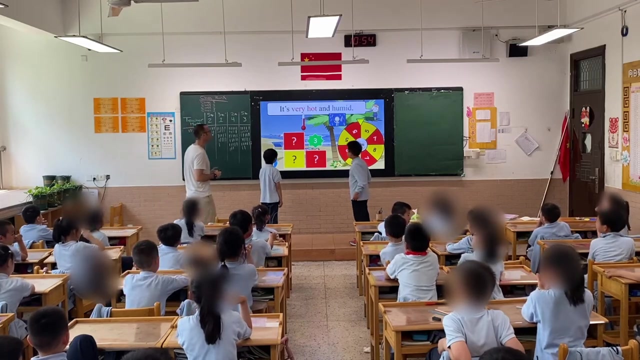 Mom, Mom, Good, How's the weather in summer? Let's see How's the weather in summer. Good, Everyone. it's very hot and humid. All right, you choose. Do you want the choosing box or just in the middle? 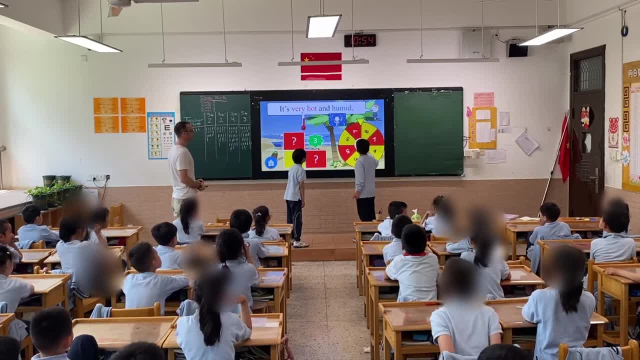 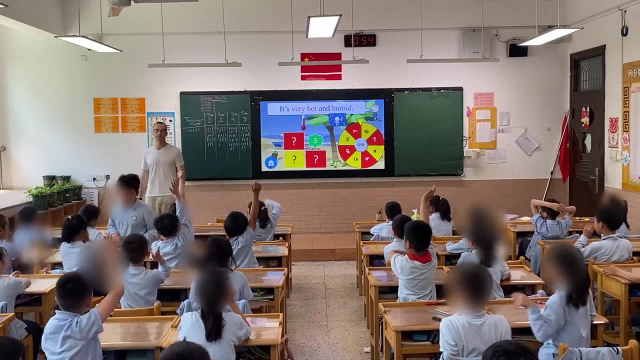 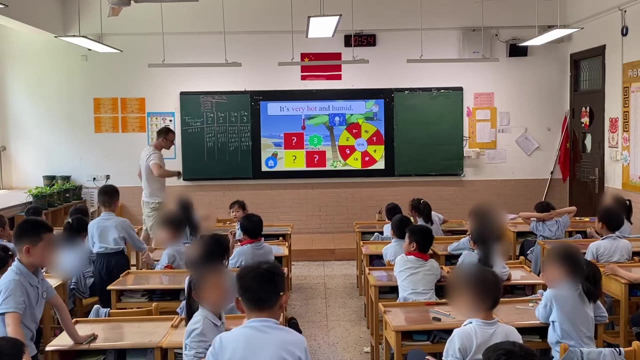 All right, it's this: one, Seven, One, two, three, four, five, six, seven. Good job. And two, one, two, one, two, one, All right. one, two, go All right. one, two, three, four. 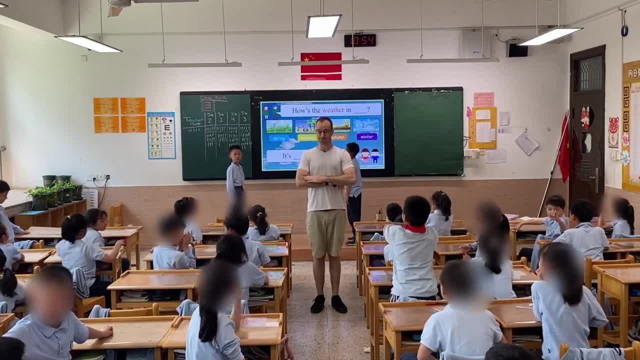 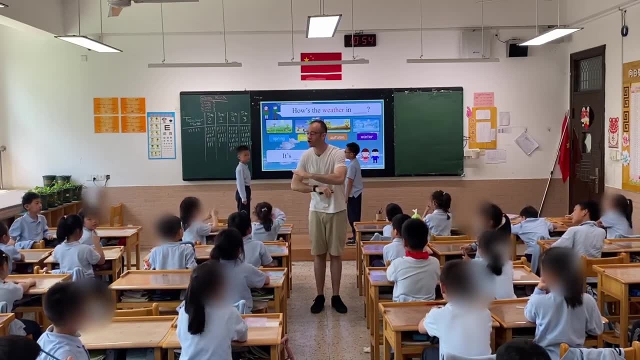 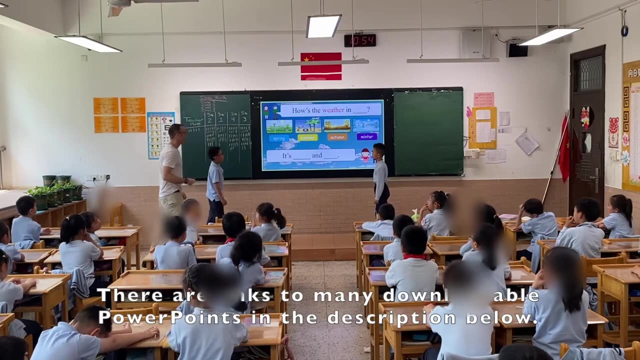 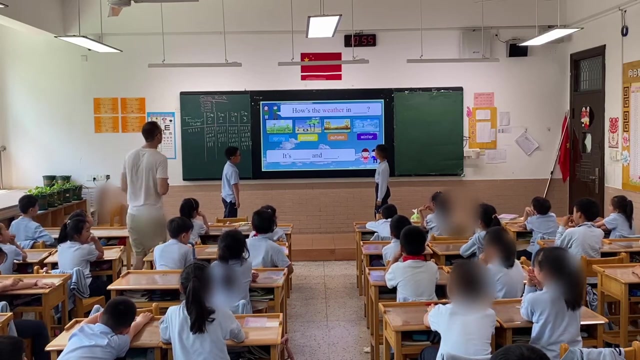 I'm going to hide my own shot for you all. All right, Class is not over. Class is not over. Sit nicely, Be quiet, Sit nicely. Thank you. All right Ready? I'll choose one. How's the weather in summer? 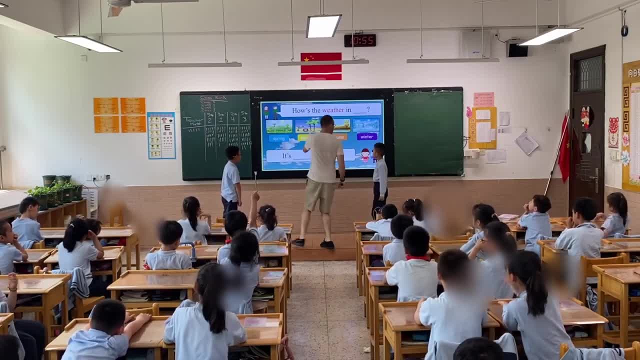 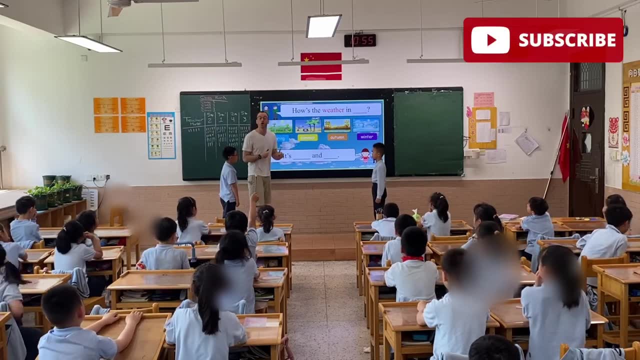 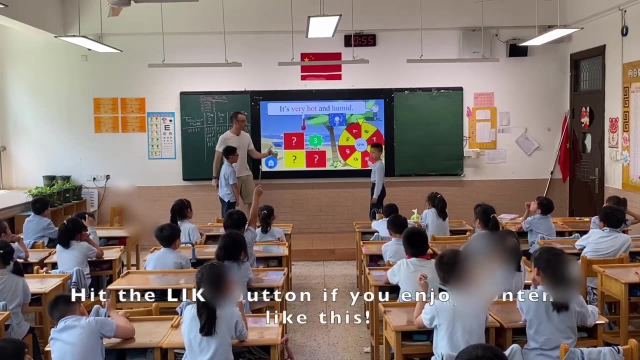 Summer: All right, How's the weather in summer, Do you remember? Okay, wet or warm. Wet, Okay, All right, choose. Do you want to spin the wheel or choose the box? All right, spin One, two, three, four, five, six, seven. 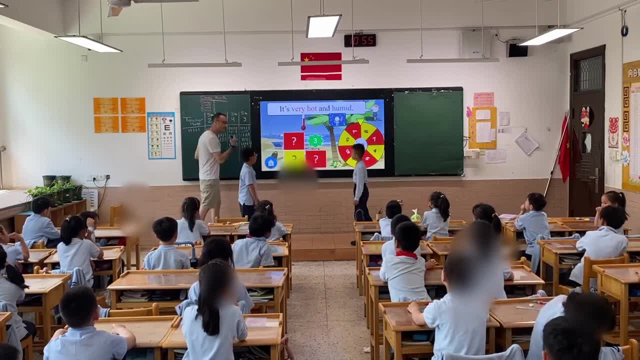 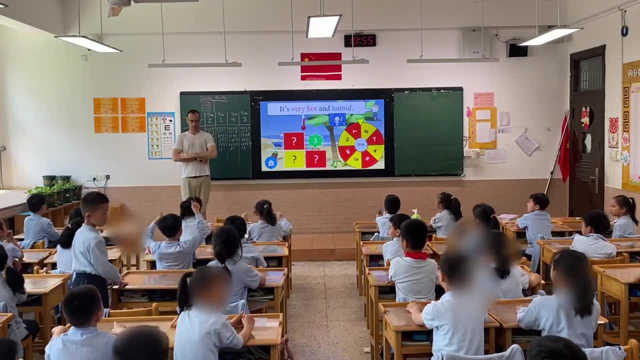 Seven, eight, nine, 10,, 11,, 12,, 13,, 14,, 15,, 16, 17.. Good job, All right. good Number five, That one's still a large chance. Let's count the score. 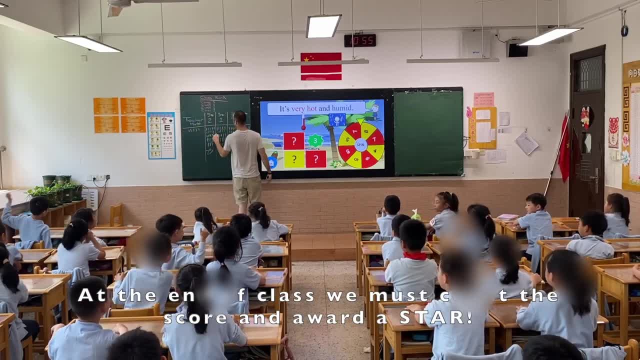 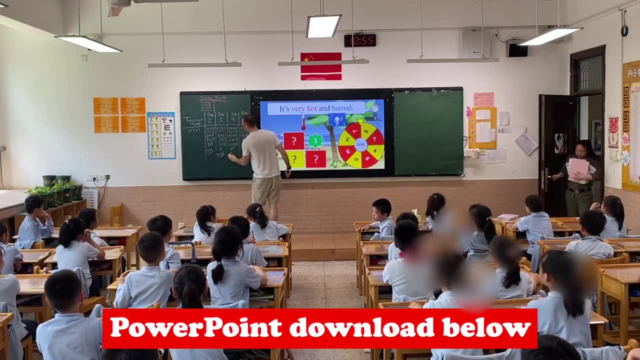 Five 10, 15,, 20, 23.. Five 10, 15,, 20, 25.. Sun's gates, Five 10, 15,, 20, 25,. ooh, Five 10,, 15,, 20, 25..